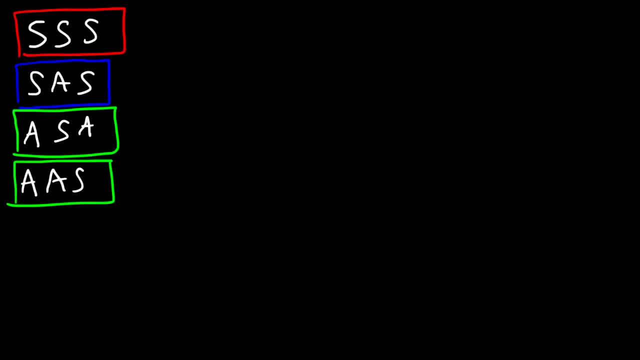 And then the last one, angle, angle side. So what I'm going to do is I'm going to give you a few triangles and I'm going to ask you which postulate applies to those two triangles that can prove that they're congruent. 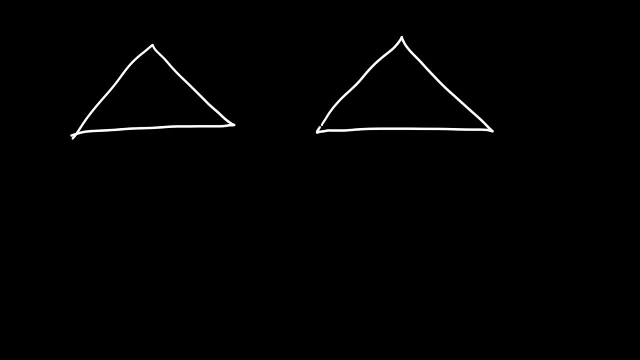 So here's the first one. So let's call this triangle ABC and triangle DEF. So let's say: if AB is congruent to DE, BC is congruent to EF and AC is congruent to DF, So what postulate proves that these two triangles are congruent? 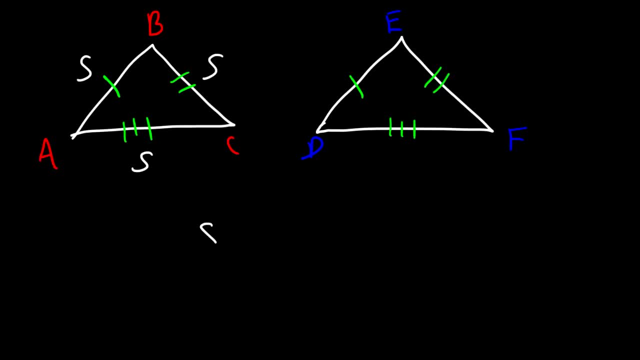 Well, we have a side, a side and another side, So we can use the SSS postulate to show that those two triangles are congruent. So we can therefore make the statement that triangle ABC is congruent to triangle DEF And make sure each letter corresponds to the same thing. 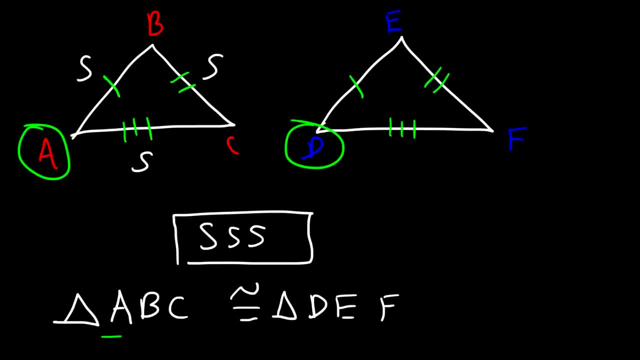 So, for example, A corresponds to D, so S be the first letter listed. B corresponds to E, so that's the same. So that's the second letter And the last one. C corresponds to F, which is the third letter. 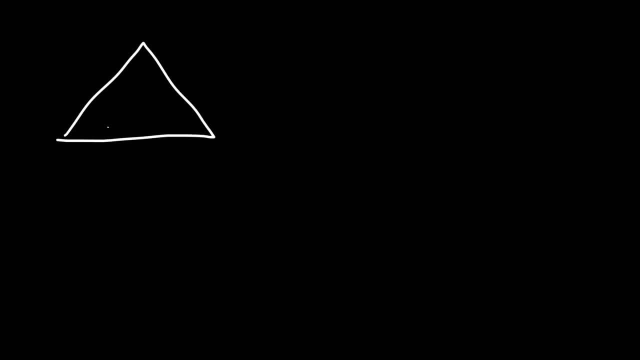 Alright. so now let's look at another example. So consider these two triangles, And let's call it triangle RST and VXY. So let's say that angle S is congruent And angle R is congruent to angle X And angle R is congruent to angle V. 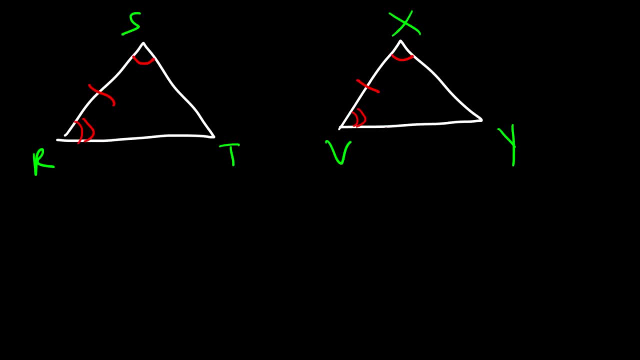 What postulate proves that these two triangles are congruent? So we have an angle, a side and an angle. You want to trace it in one direction, You don't want to jump around. So therefore we have the ASA postulate. 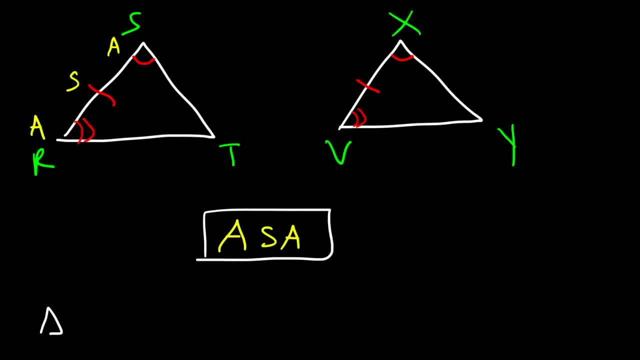 Angle side angle, And so we can make the statement that triangle RST is congruent to triangle VXY. So again, make sure that the letters match, So R corresponds to V, S corresponds to X And T corresponds to Y. 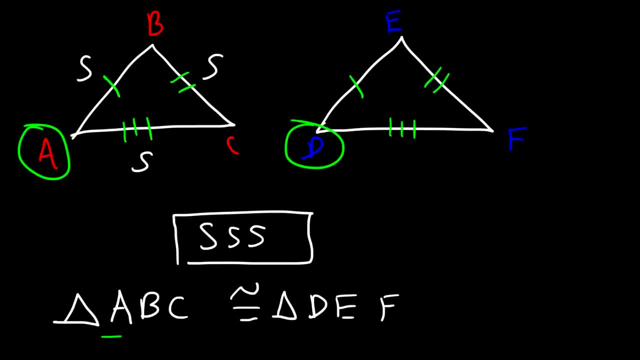 So, for example, A corresponds to D, so S be the first letter listed. B corresponds to E, so that's the same. So that's the second letter And the last one. C corresponds to F, which is the third letter. 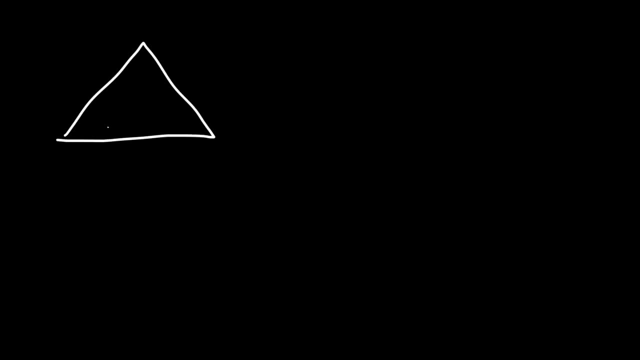 Alright. so now let's look at another example. So consider these two triangles, And let's call it triangle RST and VXY. So let's say that angle S is congruent And angle R is congruent to angle X And RS is congruent to VX. 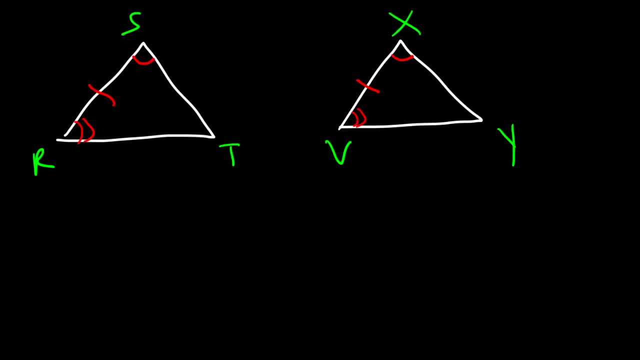 And angle R is congruent to angle V. What postulate proves that these two triangles are congruent? So we have an angle, a side and an angle. You want to trace it in one direction. You don't want to jump around. 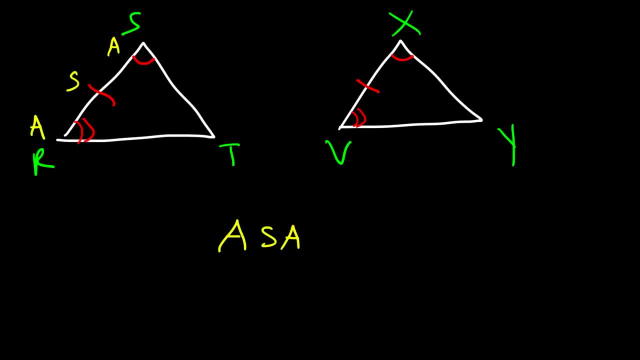 So therefore we have the ASA postulate: Angle R is congruent to angle V, Angle R is congruent to angle VXY, And so we can make the statement that triangle RST is congruent to triangle VXY. So again, make sure that the letters match. 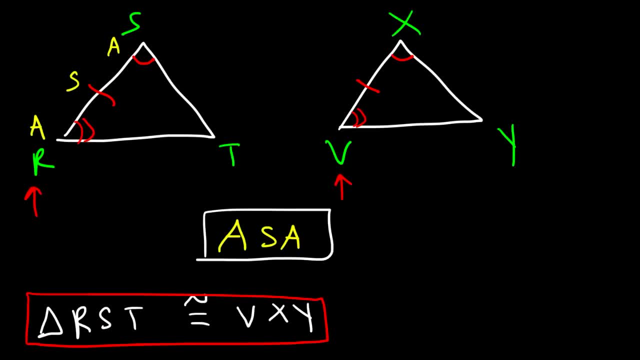 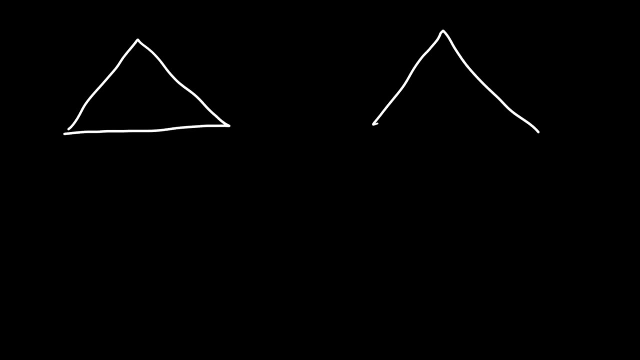 So R corresponds to V, S corresponds to X And T corresponds to Y. so let's look at another example. so let's call this triangle DEF and triangle ABC and let's say that DE is congruent to AB and DF is congruent to AC. 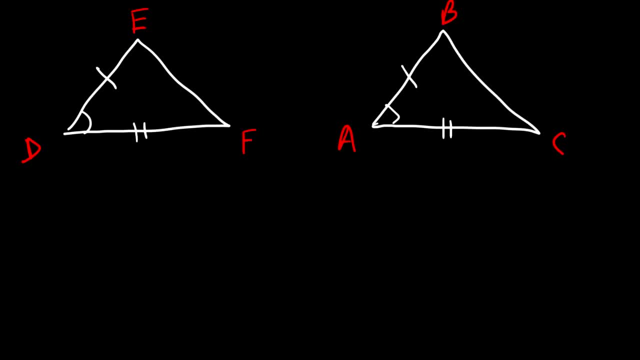 and angle D is congruent to angle A. what postulate can we use to prove that these two triangles are congruent? so we have a side, an angle and a side, so it's side angle, side SAS, and so we could therefore say that triangle DEF is congruent to. 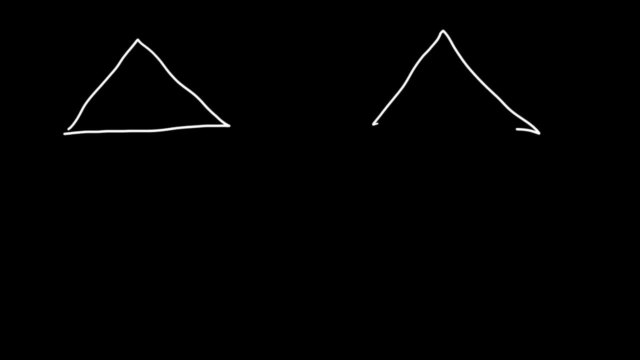 So let's look at another example. So let's call this triangle DEF and triangle ABC And let's say that DE is congruent to AB And DF is congruent to AC And angle D is congruent to angle A. What postulate can we use to prove that these two triangles are congruent? 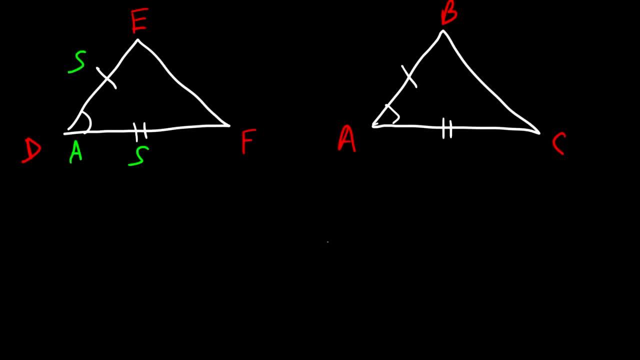 So we have a side, an angle and a side, So it's side, angle, side SAS, And so we can therefore say that triangle DEF is congruent to triangle ABC. I forgot the triangle symbol. What about this one? 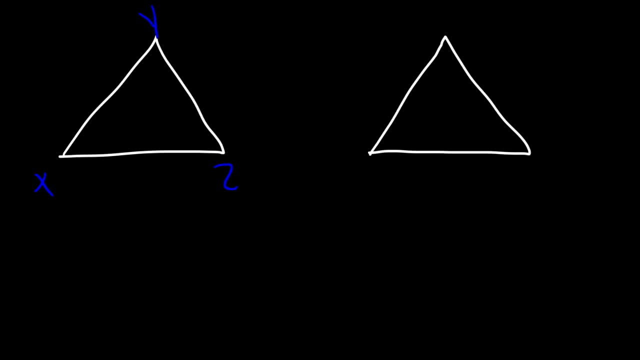 Let's call this triangle XYZ and let's say this is ABC, And let's say that XZ is congruent to AC and angle Z is congruent to angle C and angle B is congruent to angle Y. What postulate can we use to prove that these two triangles are congruent? 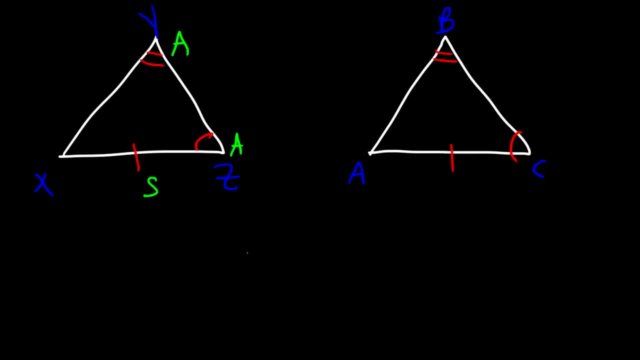 So we have an angle, an angle and a side. So by the AAS postulate these two are congruent. The triangle XYZ is congruent to triangle ABC. Now sometimes you may have a composite triangle, that is, two triangles within a single triangle. 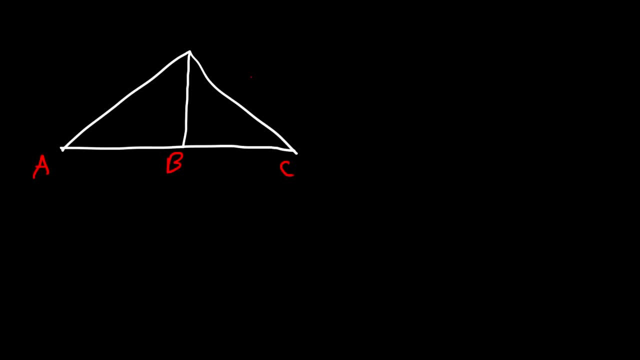 So let's say that this is A, B, C and D, And let's say that we're given that AD is congruent to CD and AB is congruent to BC. Okay, Okay, Okay, Okay, Okay Okay. 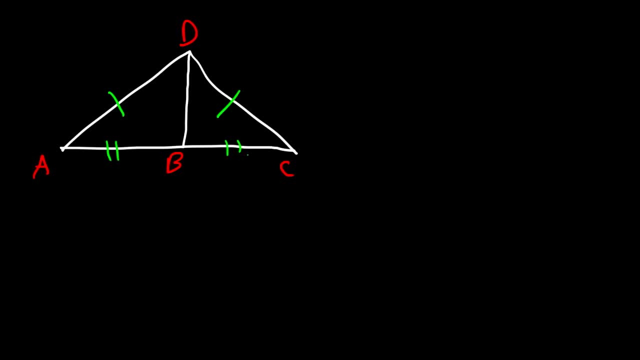 What can we prove? What conclusions can we draw? So let's separate this composite triangle into two triangles. So the first one on the left is triangle ABD. On the right, we have triangle CBD. So we know that AD and DC are the same. 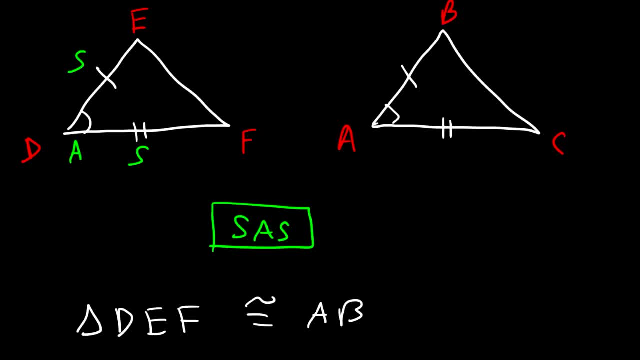 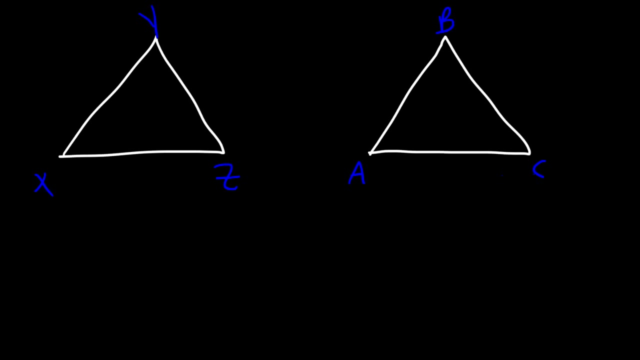 triangle ABC and I forgot the triangle symbol. what about this one? let's call this triangle XYZ and let's say this is ABC. and let's say that XZ is congruent to AC and angle z is congruent angle see an angle B is congruent angle Y. 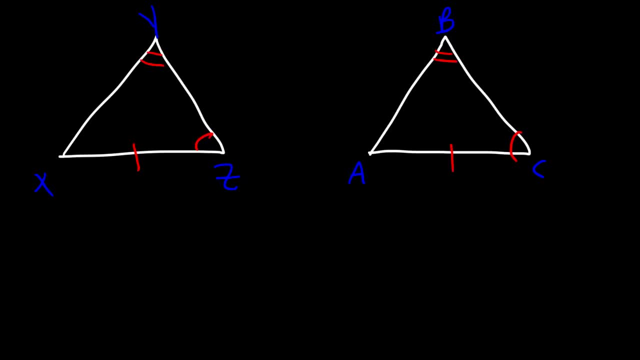 well, partially, can we use prove that these two triangles are congruent. so we have an angle and angle and aside. so by the AAS, possibly these two are congruent. the triangle XYZ is congruent to triangle ABC. yes, you may have a composite triangle, that is, two triangles within a single. 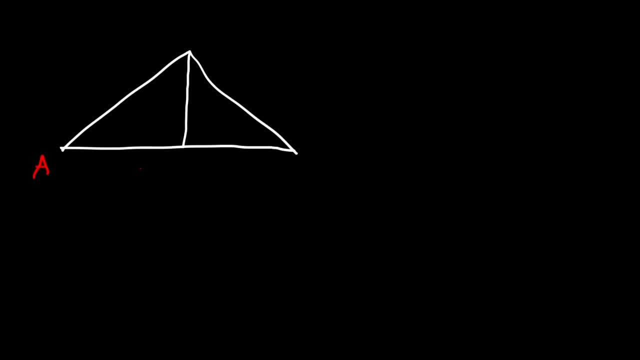 triangle. so let's say that this is a, B, C and D. now let's say that we're given that ad is congruent to CD and a- B is congruent to BC. what can we prove? what can we? what conclusions can we draw? so let's separate this composite triangle. 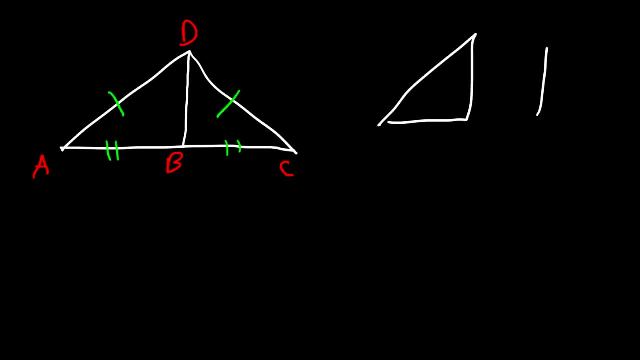 into two triangles. so the first one on the left is triangle a- B D. on the right, we have triangle C- B- D. so we know that ad and DC are the same, a, B and BC are the same, but notice that they share a common sequence of triangles. so we know that a, B and BC are the same, but notice that. 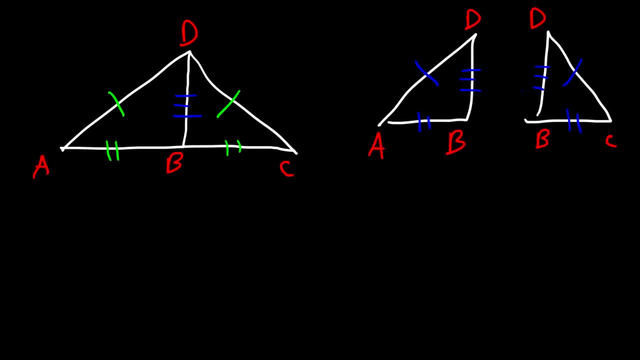 side, and that is DB, is equal to DB because that's the same segment. so therefore we have two triangles that share to have the same three sides. so these two triangles are congruent by the SSS partially. so sometimes if you don't see the two triangles, you may want to split this composite triangle into two. 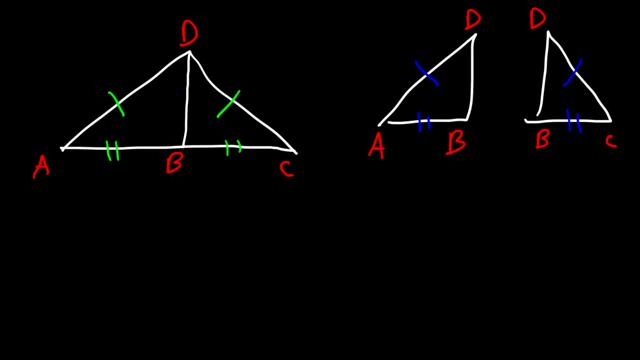 AB and BC are the same, But notice that they share a common side and that is DB is equal to DB because that's the same segment. So therefore we have two triangles that share, that have the same three sides. So these two triangles are congruent by the SSS postulate. 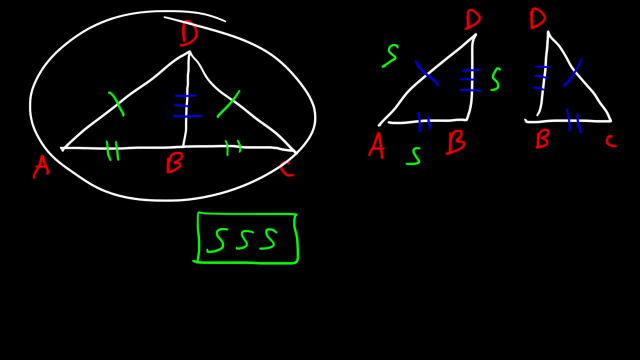 So sometimes, if you don't see the two triangles, you may want to split this composite triangle into two smaller triangles, if that helps. So we can make the statement that AB and BC are congruent And this gives us the statement that triangle ABD is congruent to triangle CBD. 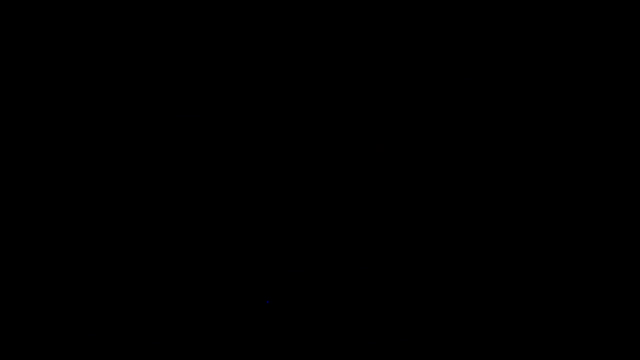 I can show again the triangle. ABD is congruent to triangle CBD. Okay, So let's try another composite figure. Let's call this ABCDE. So let's say that in this case, ABD is congruent to triangle CBD. 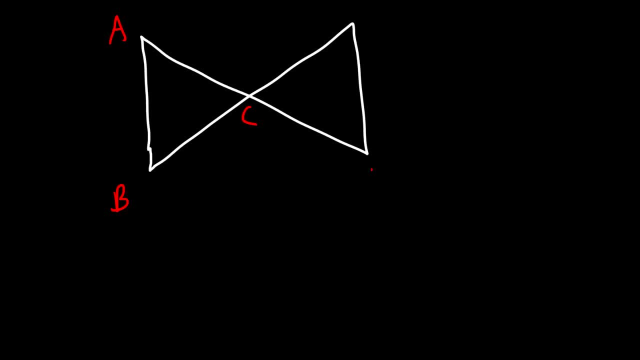 So what that means is that, in this case, ABD is congruent to triangle CBD, It's congruent, AC is congruent to EC and also angle A is congruent to angle E. What can we do to prove that the two triangles are congruent? The triangle on the left- ACB. 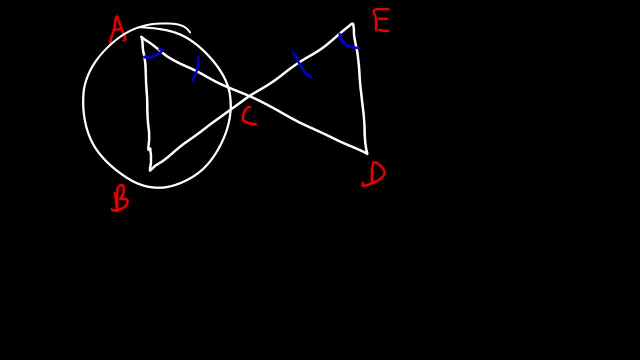 and the triangle on the right, ECB. Right now, we only have two things that are congruent. We have an angle and a side. Is there anything else that we could see that's congruent? Now, whenever you have two lines that intersect each other or 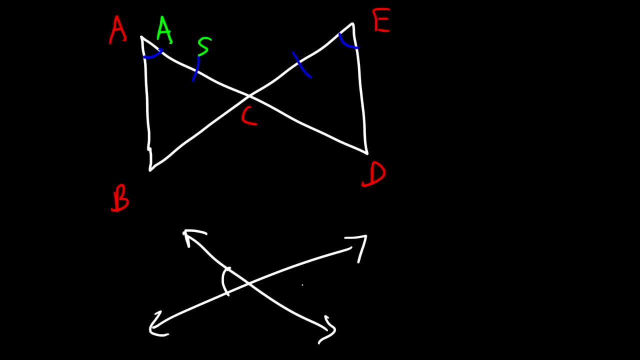 two segments, they will produce something known as vertical angles. Vertical angles are congruent. So in this picture angle 1 is congruent to angle 2 and 3 is congruent to angle 4.. So therefore angle ACB is congruent to ECD. 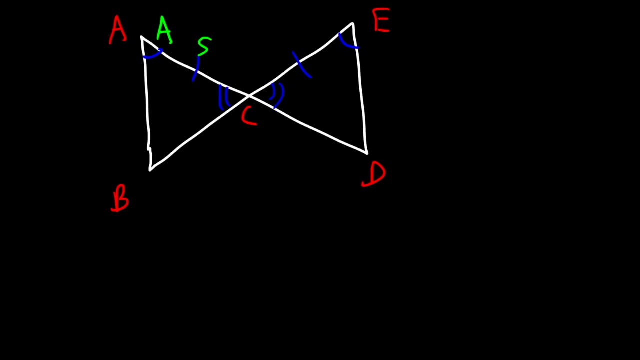 And we now could prove that the two triangles are congruent by the ASA postulate. So we have two angles and the side between the two angles. So now we can say that triangle ACB is congruent to triangle ECD. Notice that E and A. 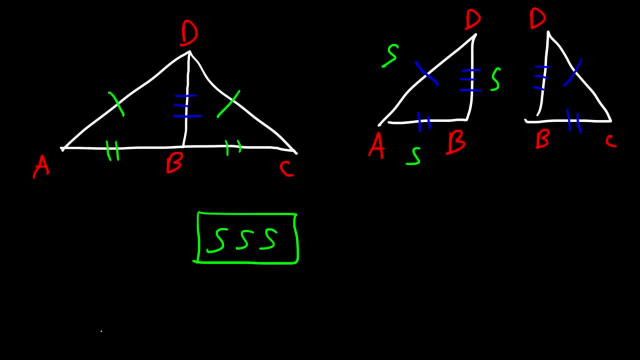 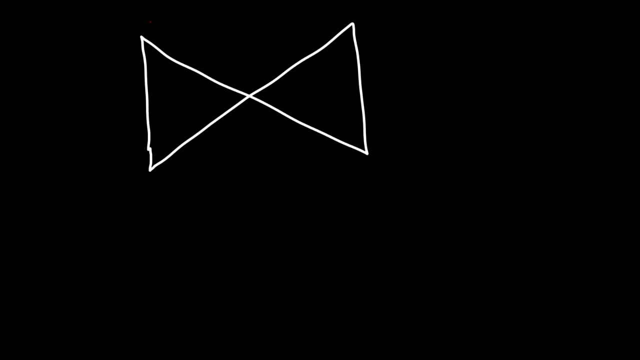 smaller triangles, if that helps. so we can make the statement that triangle a, B, D is congruent to triangle C, B, D. let's try another composite figure. let's call this a, B, C, D and E. so let's say that AC is congruent to EC and also a. 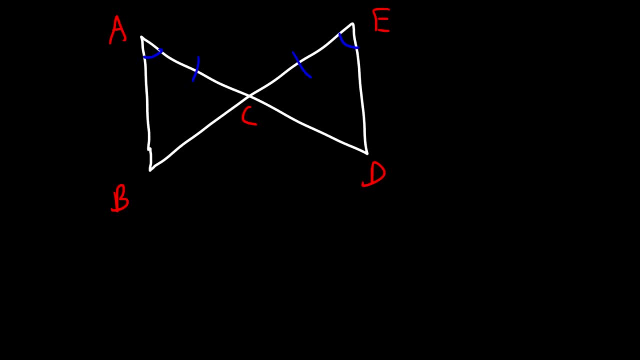 angle a is congruent to angle e. what can we do to prove that the two triangles are congruent? the triangle on the left, ACB, and the triangle on the right, ECB. right now, we only have two things that are congruent: we have an angle and a side is. 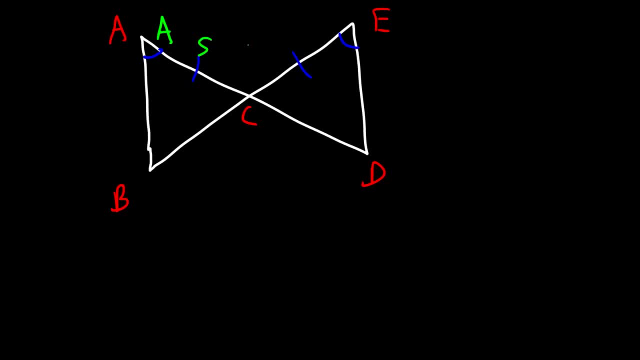 there anything else that we could see that's congruent? now, whenever you have two lines that intersect each other, or two segments, they will produce something known as vertical angles. vertical angles are congruent, so in this picture, angle one is congruent to angle 2 and 3 is congruent to angle 4, so therefore angle: 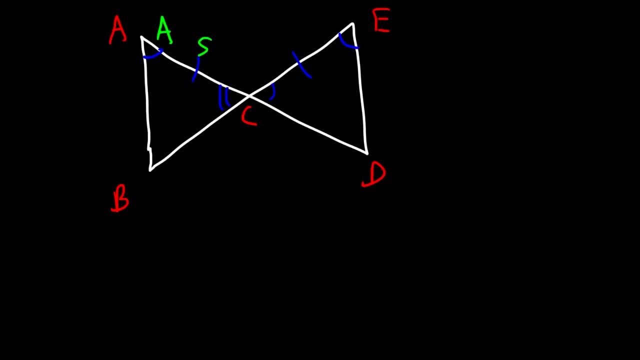 a CB is congruent to E, CD, and we now could prove that the two triangles are congruent by the ASA porta- droite angle A, C, or the angle point A is congruent to A, S, D, and we now could prove that the two triangles are congruent by the ASA, partly the same but relatively same Mattige Angle, one with coaxing angles is congruent, or two articles are congruent: a vertical lines. 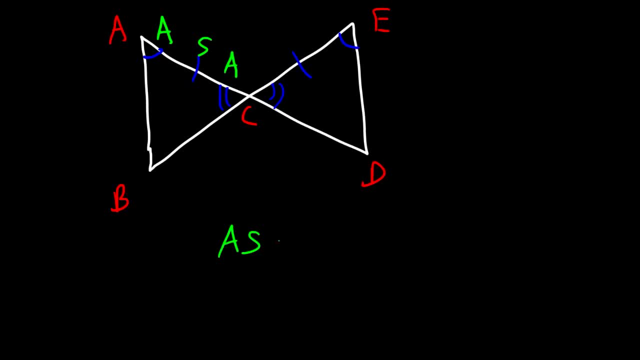 postulate. So we have two angles and the side between the two angles. So now we can say that triangle ACB is congruent to triangle ECD. Notice that E and A are the same in this particular example and D and B correspond to each other. 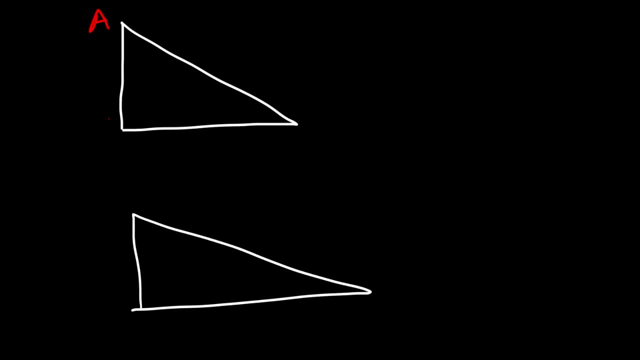 So let's say that this is triangle ABC and triangle DEF. Now let's say that angle A is congruent to angle D and that angle B is congruent to angle E and angle C is congruent to angle F. So are these two triangles congruent? So we have an. 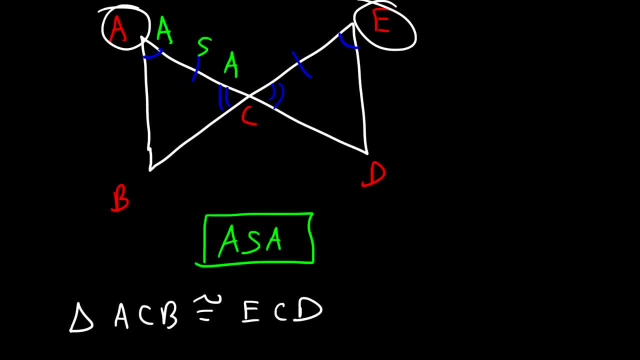 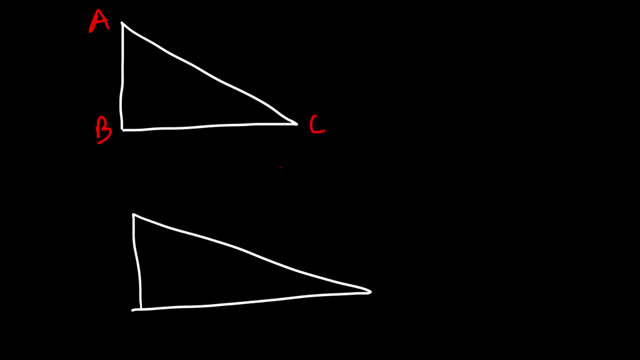 are the same in this particular example and D and B correspond to each other. So let's say that this is triangle ABC and triangle DEF. Now let's say that angle A is congruent to angle D and that angle B is congruent to angle E and angle. 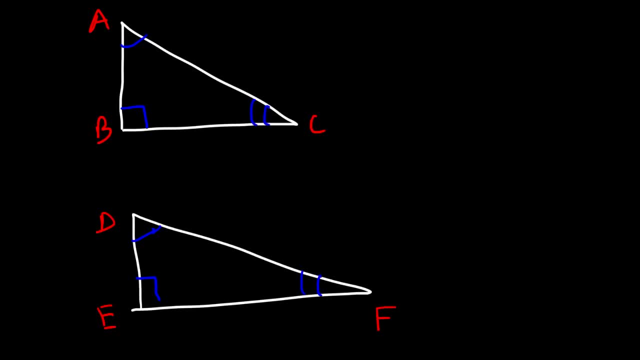 C is congruent to angle F, So are these two triangles congruent. So we have an angle, an angle and an angle. So is there such a postulate, the AAA postulate? No, there isn't. So therefore these two triangles are not congruent. So we can write this statement: Triangle ABC. 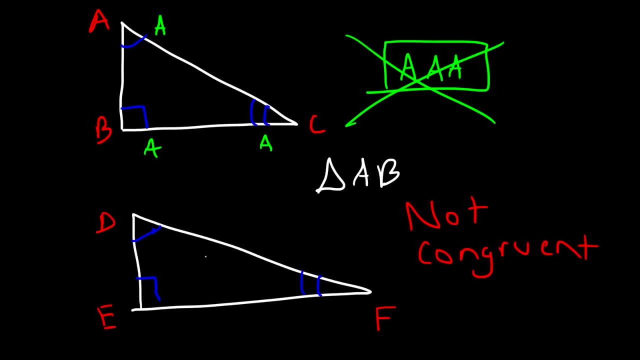 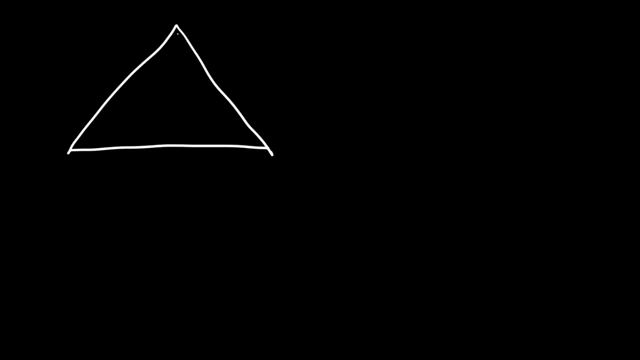 I put S for some reason. Let's correct that It is not congruent to triangle DEF. So let's say this is XYZ, Let's call this A And in this example we're going to say that angle X is equal to angle Z. 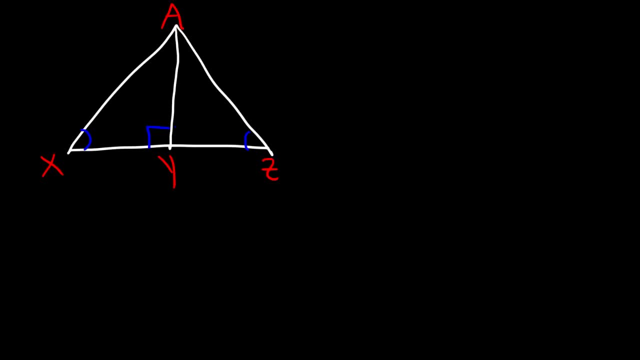 And XYA is congruent to ZYA. And with this information, what can we conclude about these two triangles? Can we say that triangle XYA is congruent to triangle ZYA? Now, remember, they share a common side. That is YA. So we could say: 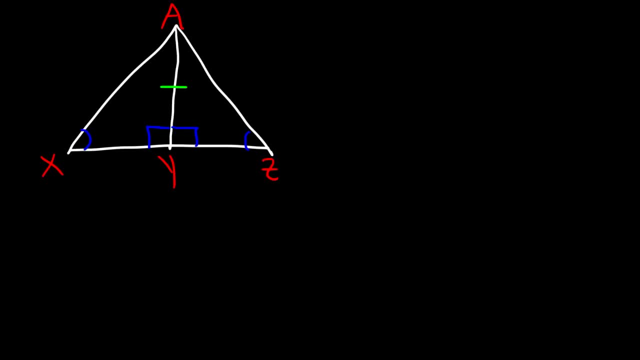 that YA is congruent to YA for the two small triangles based on the reflexive property. Thus we have an angle, an angle and a side. So by the AAS postulate, which is one of the four that we mentioned in the beginning, these two triangles are: 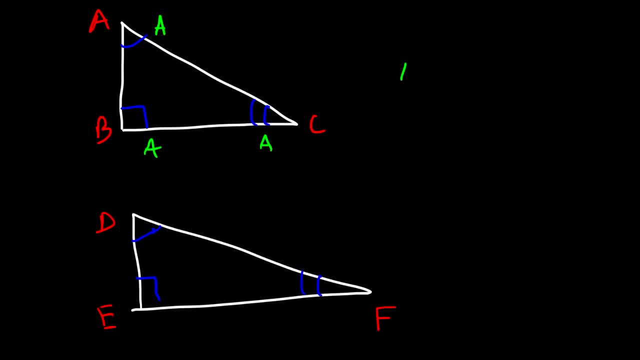 angle, an angle and an angle. So is there such a postulate, the AAA postulate? No, there isn't. So therefore these two triangles are not congruent. So we can write this statement: Triangle ABC. I put S for some reason. let's correct, that is not. 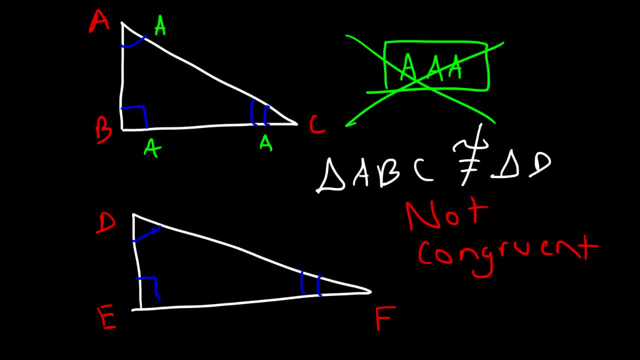 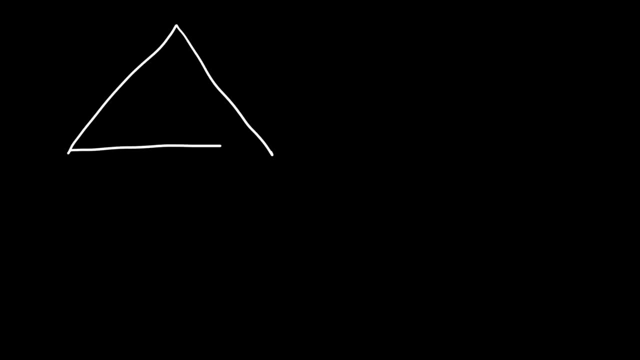 congruent to triangle DC, Triangle ACB is congruent to triangle DEF. So let's say this is X Y Z, let's call this A And in this example we're going to say that angle X is equal to angle Z and X Y A is congruent to Z Y A. 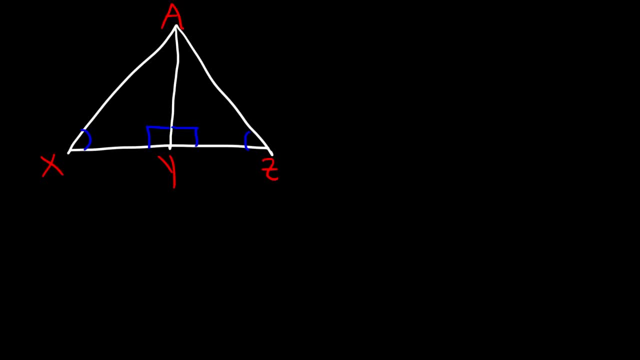 and with this information, what can we include about these two triangles? can we say that triangle X, Y a is congruent to triangle Z, YA? now remember, they share a common side. that is why a. so we could say that why a is congruent to, why a for. 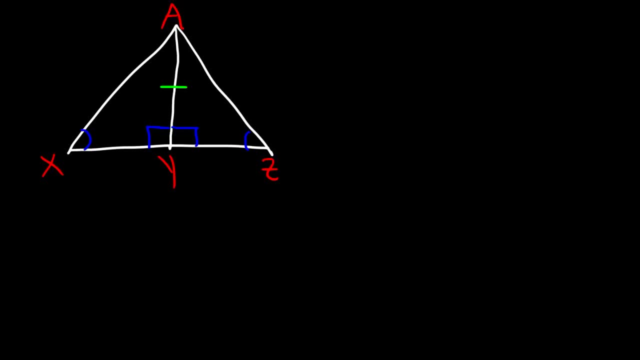 the two small triangles based on a reflexive property. thus we have an angle and angle and a side. so by the AAS postulate, which is one of the four that we mentioned in beginning, these two triangles are congruent. it's a triangle X, Y. a is congruent to triangle Z, YA. 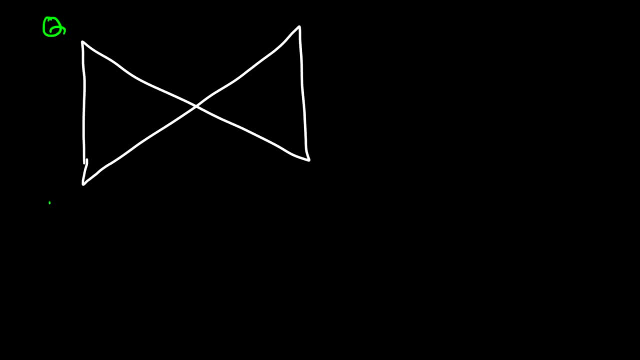 so let's say this is q are sst. let's say X, i, let's say that qs is congruent to st and RS is congruent to x, proved that these two triangles are congruent. so, as you recall, angle R, sq is a vertical angle. with XST, those tour vertical angles, which means 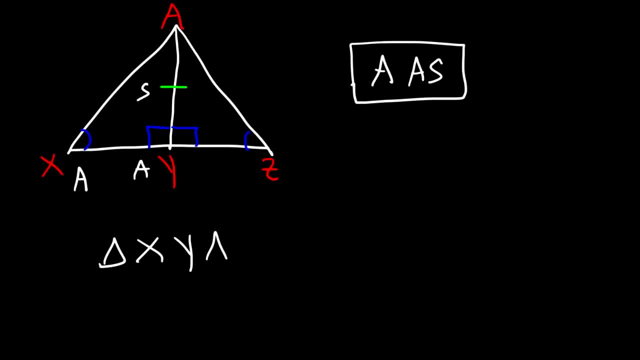 congruent. So triangle XYA is congruent to triangle ZYA. So let's say this is QRST, let's say X And let's say that QS is congruent to ST and RS is congruent to SX. Prove that these two triangles are congruent. So, as you recall, angle RSQ is a vertical. 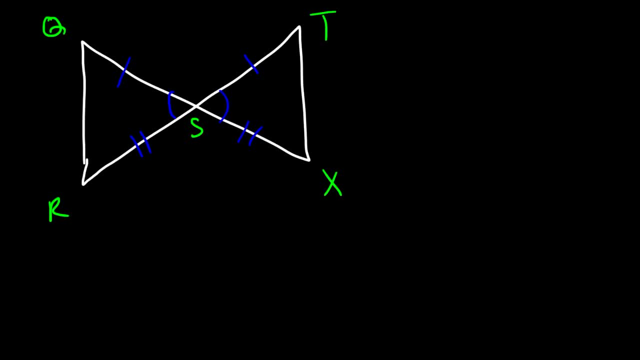 angle X, S, T. Those two are vertical angles, which means that they're congruent. So we have a side, an angle and a side. So by the SAS postulate we can say that triangle R, S, Q 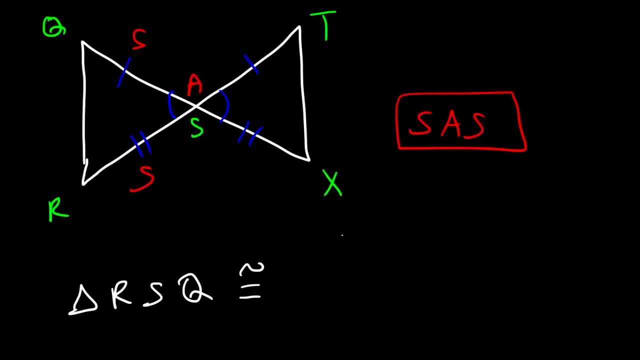 is congruent to triangle X S T. So notice that R and X are opposite to the same side. So therefore R and X are congruent And T is opposite to the same side as Q, So Q and T are congruent. So therefore, triangle R S Q is congruent to triangle X S T. 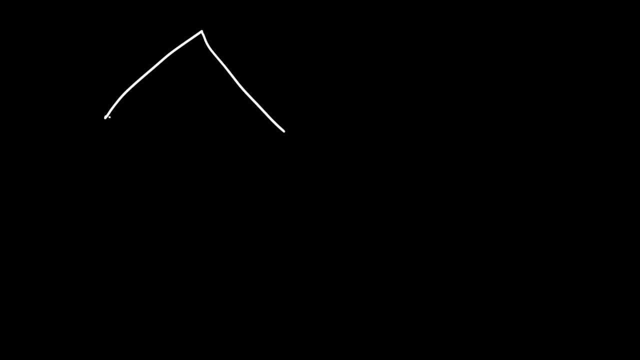 Now let's look at one last example before we work on two column proofs. Let's call this A, B, C and D, And let's say that AB is congruent to AD and BC is congruent to DC. What do we need in order to prove that these two triangles are congruent? 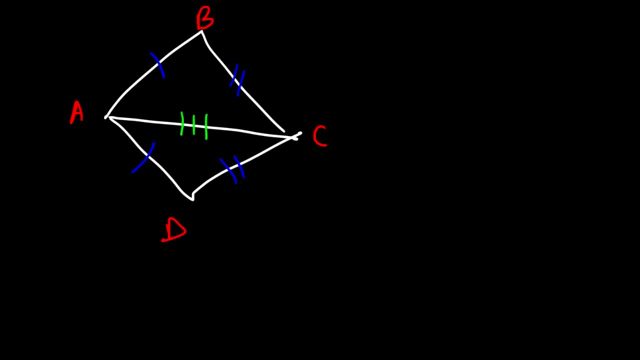 Now they share the same side, side AC. So therefore we have a side side and a side. So by the SAS postulate we can say that triangle ABC is congruent to triangle ADC. And that's it. Now let's work on some two column proofs. 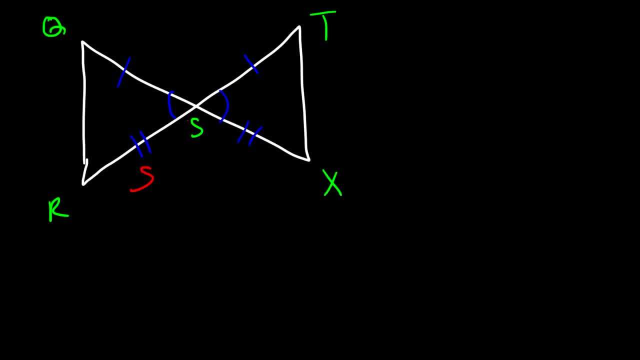 that there can congruent. So we have a side, an angle and a side. So by the SAS postulate we can say that triangle RSQ is congruent to triangle XST. So notice that R and X are opposite to the same. 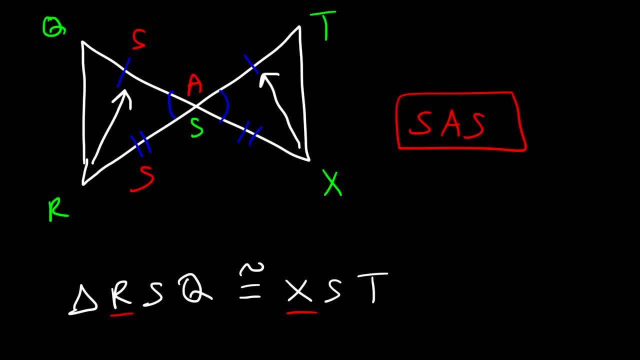 side. So therefore R and X are congruent And T is opposite to the same side as Q. So Q and T are congruent. So therefore, triangle RSQ is congruent to triangle XST. Now let's look at one last example before we work on. 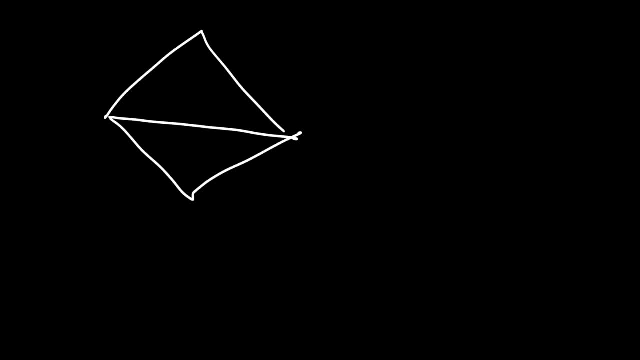 two-column proofs. Let's call this A, B, C and D. Now let's say that A B is congruent to A D and B C is congruent to D- C. What do we need in order to prove that these two triangles are? 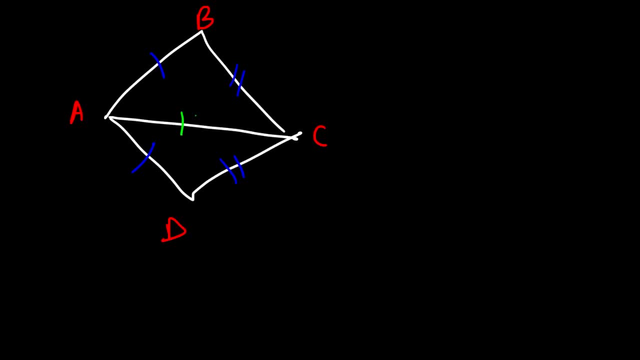 congruent. Now they share the same side, side AC. So therefore we have a side side and a side. So by the SAS postulate we can say that triangle RSQ is congruent to triangle XST. So by the SAS, 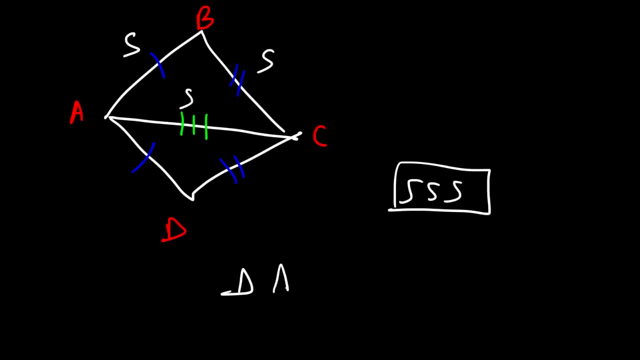 SS postulate we can say that triangle ABC is congruent to triangle ADC and that's it. Now let's work on some two-column proofs. Let's say this is A, B, C and D, and we're given that segment AD is congruent to CD. 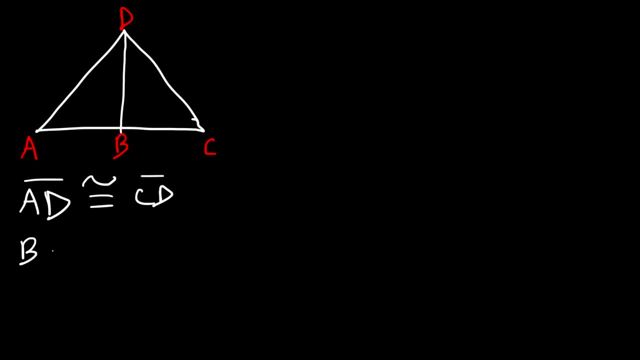 and also that B is the midpoint of AC. Your task is to prove that the two triangles are congruent, That triangle ABD is congruent to triangle CBD. So feel free to pause the video if you want to. So let's write our two columns. 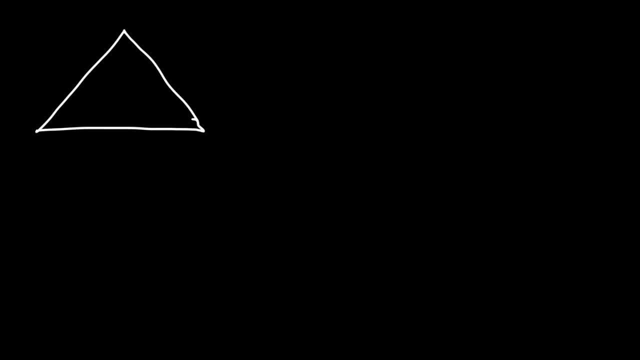 Let's say this is A, B, C and D, And we're given that segment AD is congruent to CD, But also that B is the midpoint of AC. Your task is to prove that the two triangles are congruent, That triangle ABD is congruent to triangle CD. 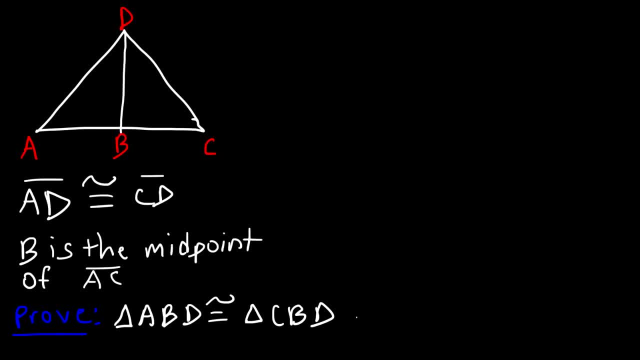 So feel free to pause the video if you want to. So let's write our two columns: statements and reasons. So the first thing you should do, as always, is rewrite what you're given So we know that AD is congruent. 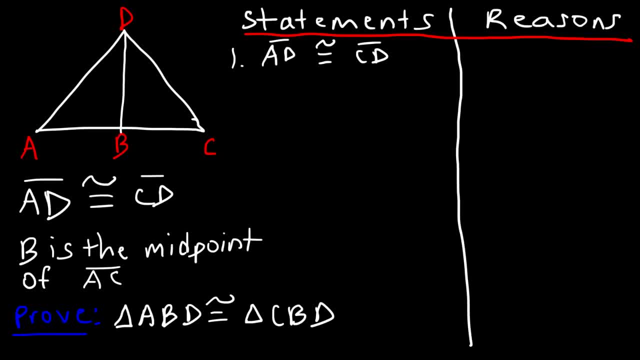 To CD And that's a given, And we know that B is the midpoint. Let me just mark that AD is congruent to CD. Now B is the midpoint of segment AC, So that's given. Now, what are some conclusions that we can draw if B is the midpoint? 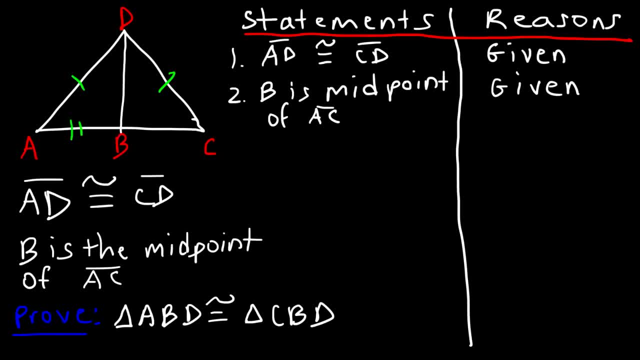 Okay, If B is the midpoint, that means that AB is congruent to BC. So let's write that in step three. So AB is congruent to BC And the reason: Definition of a midpoint. Now, let's get rid of this stuff. 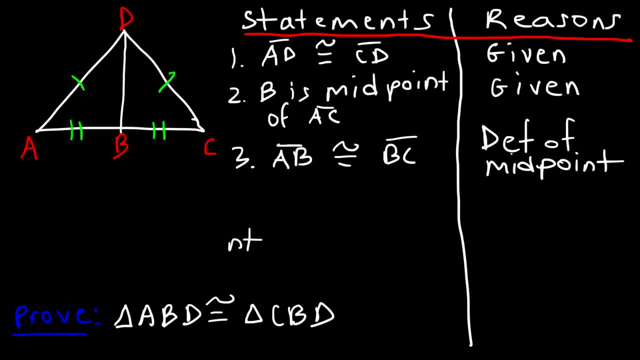 It's just taking up space. Okay, So let's write B. So we look at that. Now, what else can we say? So right now, we have two sides. We either need another angle or another side. Now notice that BD is shared between both triangles. 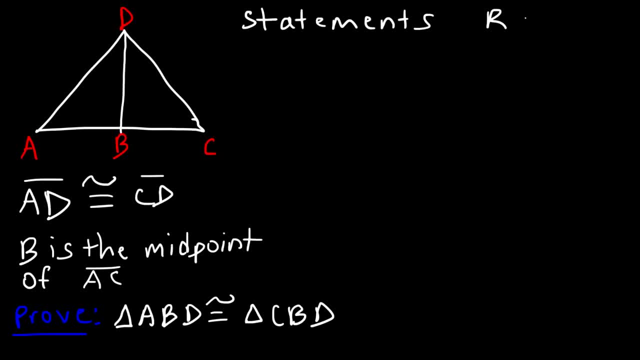 statements and reasons. So the first thing you should do, as always, is rewrite what you're given. So we know that AD is congruent to CD, and that's a given, And we know that AD is congruent to CD and we know that B is the midpoint. 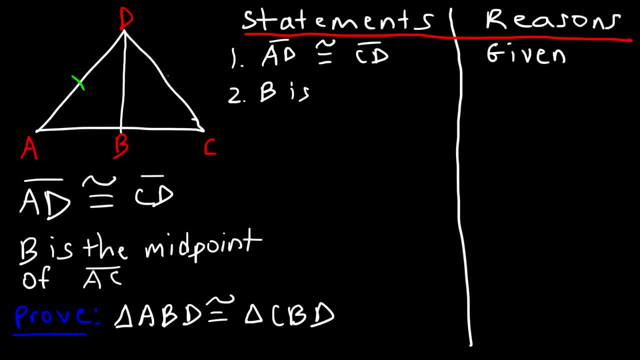 But let me just mark that AD is congruent to CD. Now B is the midpoint of segment AC. So that's given. Now, what are some conclusions that we can draw? if B is the midpoint, If B is the midpoint, that means that AB is congruent to BC. 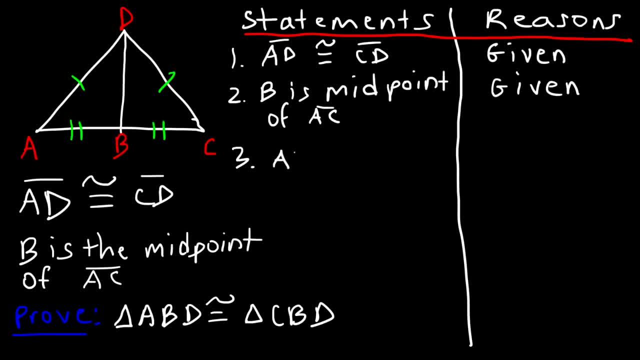 So let's write that in step three. So AB is congruent to BC And the reason: Definition of a midpoint. Now, let's get rid of this stuff. It's just taking up space. Now, what else can we say? 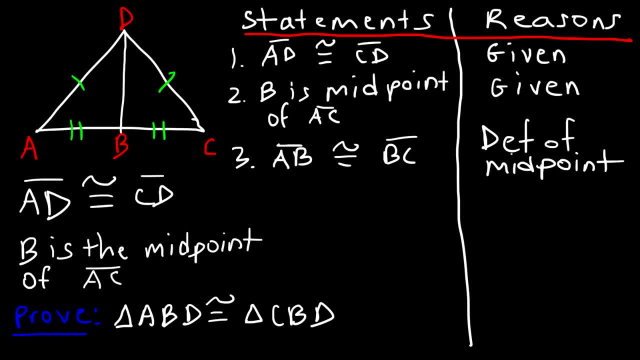 If B is the midpoint of segment AC, that means that AB is congruent to CD and that's a given. So let's write that in step three. So AB is congruent to BC. And the reason: Definition of a midpoint. 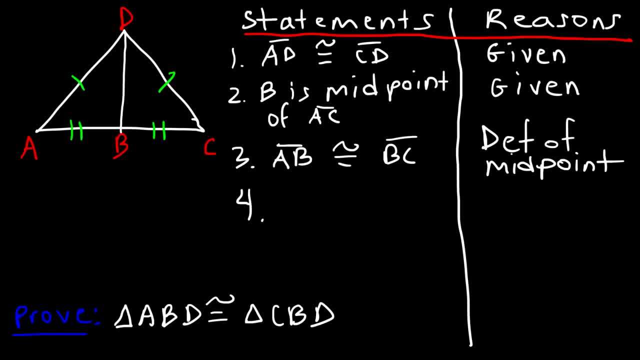 Now let's get rid of this stuff. It's just taking up space. So right now we have two sides. We either need another angle or another side. Now notice that BD is shared between both triangles. So that's the third side. 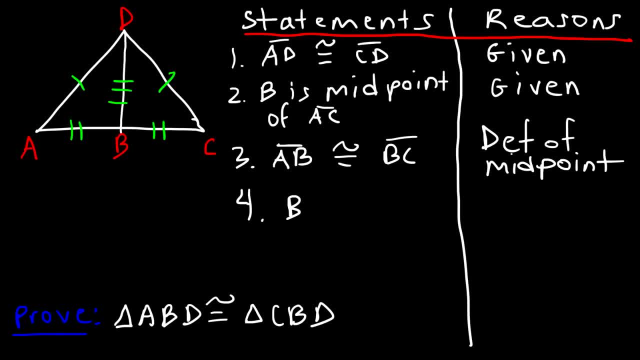 That's the common side, So we could say that BD is congruent to itself. And whenever you have a common side, the reason you can always write is the reflexive property. Now, let's get rid of this stuff. Now, what postulate can we use to prove that these two triangles are congruent? 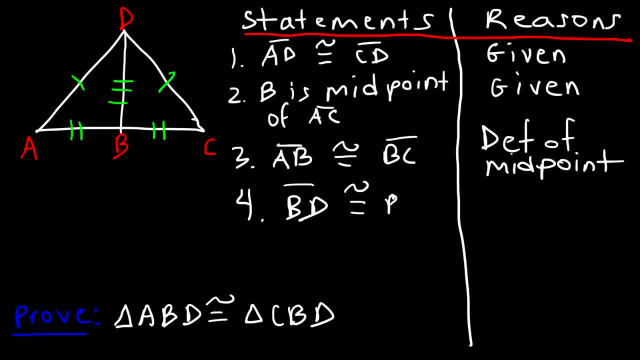 So that's the third side, That's the common side. So we could say that BD is congruent to itself. The reason you can always write is the reflexive property. Now what postulate can we use to prove that these two triangles are congruent? 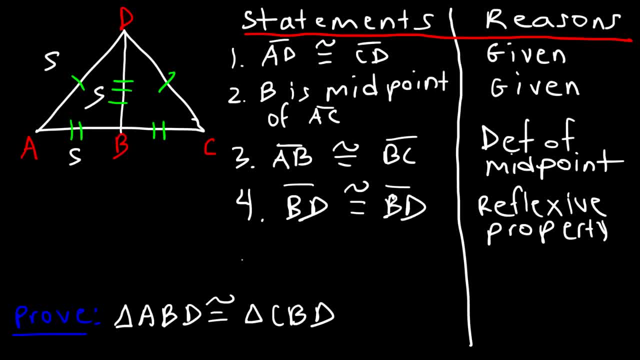 So notice that we have a side, a side and another side, So we can make the final statement that triangle ABD is congruent to triangle CBD And the reason for that is the SSS postulate, And we're using statements 1 that show that these two sides are congruent. 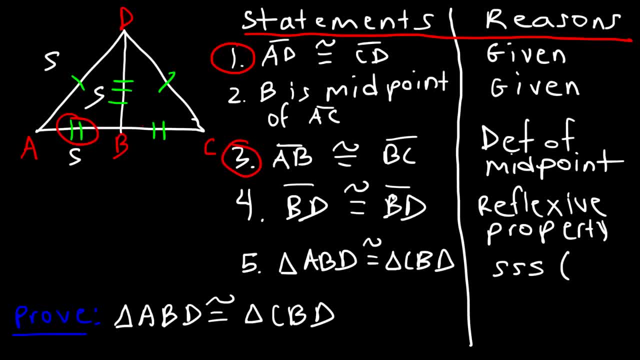 And statement 3,, which show that AB is congruent to BC, And also statement 4, where BD is congruent to itself, And so we're going to write 1, 3, S And 4.. And so that's how you can prove that two triangles are congruent. 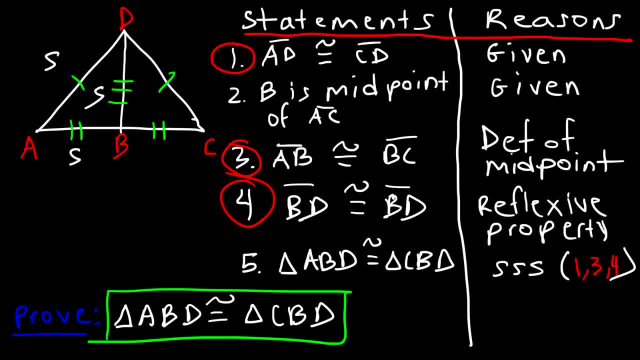 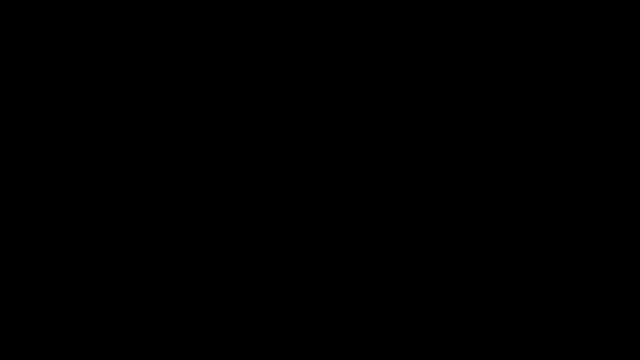 You can use the SSS postulate, SAS, ASA or AAS. By the way, I recommend that you pause the video for each of these problems, And it's best if you work on it, because that's the way you're going to learn. 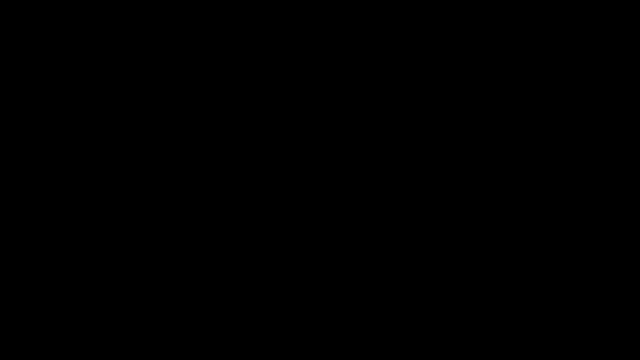 Pause the video, try the problem and then, once you get the answer, unpause it to see the solution. Okay, So you might have a different way of getting to the answer. So sometimes there's more than one way. So I just want to let you know about that. 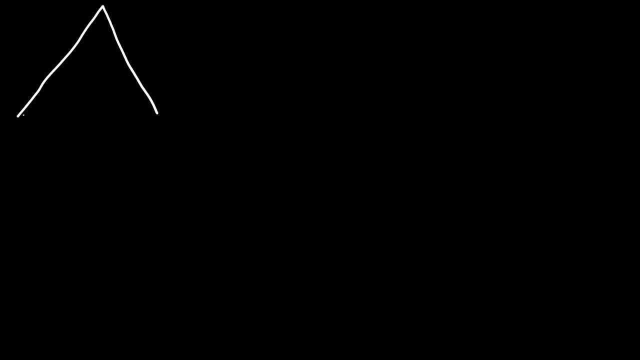 Now let's go ahead and begin. So let's call this MOP And this is going to be R And we're given that segment RO, It's perpendicular to segment MP And also segment MO is congruent to segment OP. 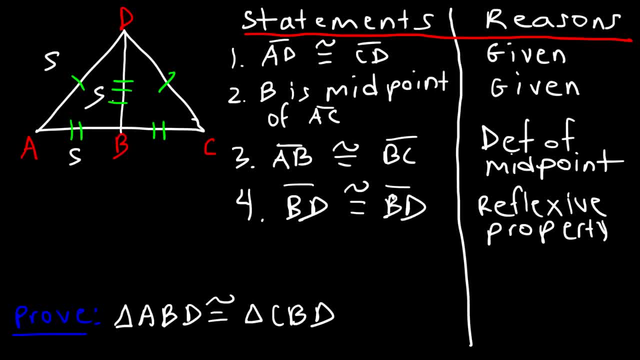 So notice that we have a side, a side and another side, So we can make the final statement that triangle ABD is congruent to triangle CBD And the reason for that is the SSS postulate, And we're using statements 1. 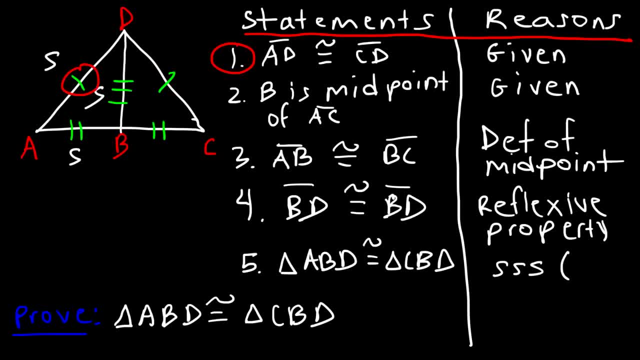 that show that these two sides are congruent, And statement 3, which show that AB is congruent to BC, And also statement 4, where BD is congruent to itself, And so we're going to write 1,, 3, and 4.. 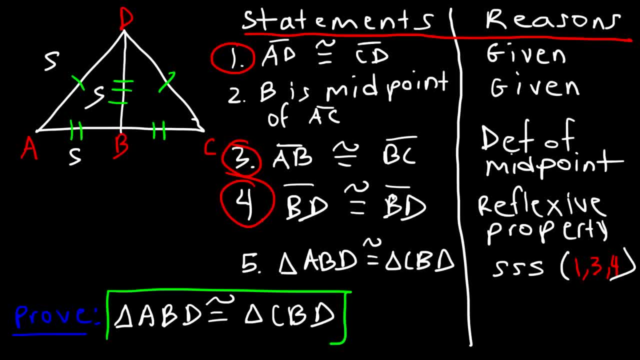 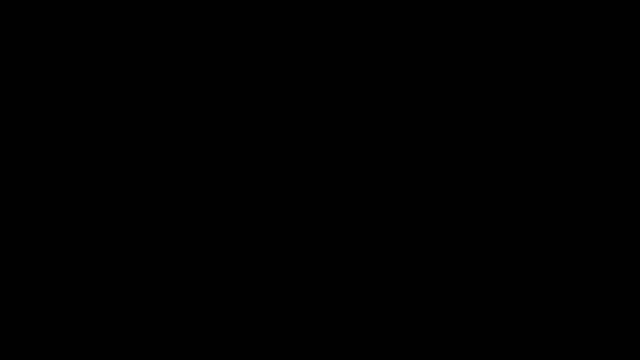 And so that's how you can prove that two triangles are congruent. You can use the SSS postulate as a or ASA. By the way, I recommend that you pause the video for each of these problems, And it's best if you work on it. 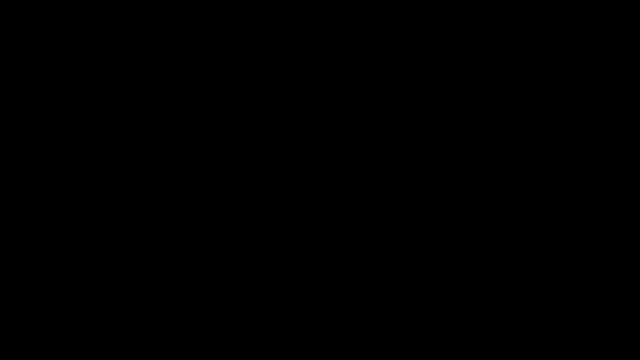 Because that's the way you're going to learn. Pause the video, try the problem and then, once you get the answer, unpause it to see the solution. Now you might have a different way of getting to the answer, so sometimes there's more than one way. 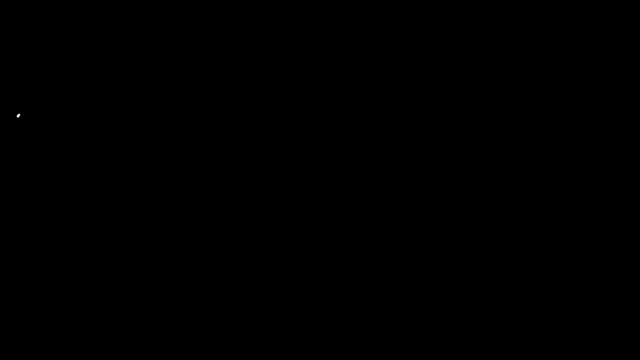 So just wanna let you know about that. Now let's go ahead and begin. So let's call this MOP, So let's call this MOP, So let's call this MOP, and this is going to be R, and this is going to be R. 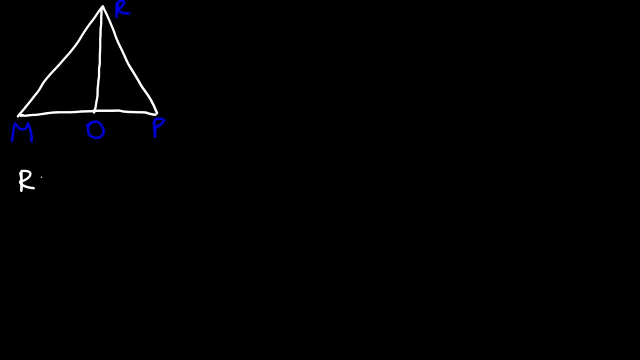 And we're given that segment RO is perpendicular to segment MP, to segment MP, And also segment MO is congruent to segment OP. Your task is to prove that triangle MRO is congruent to triangle PRO. So go ahead and begin, See if you can do this. 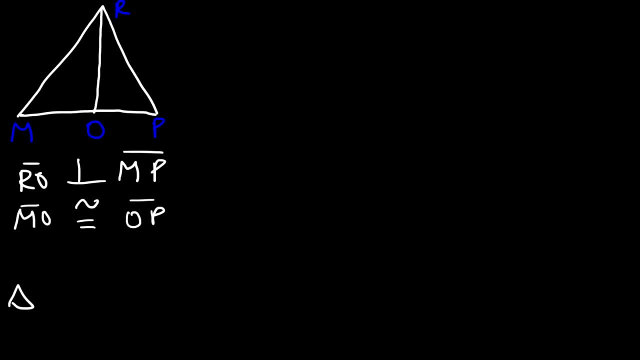 Your task is to prove that triangle MRO is congruent to triangle PRO, So go ahead and begin, See if you can do this. So let's write our two-column proof. So, as always, what's the first thing that we should do? 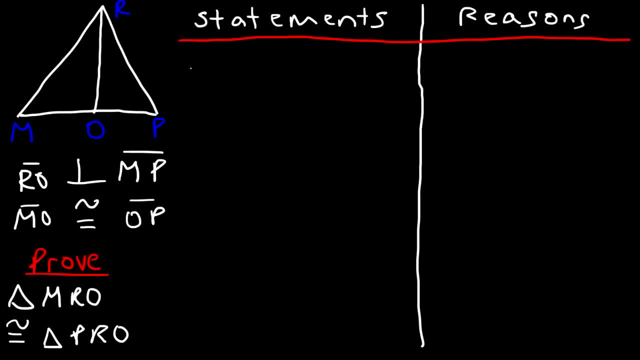 Remember, the first thing you should do is write the given. So first let's start with the fact that Segment MO is congruent to segment OP and that's given. And just to keep things in perspective, just to make it easier, let's highlight that. 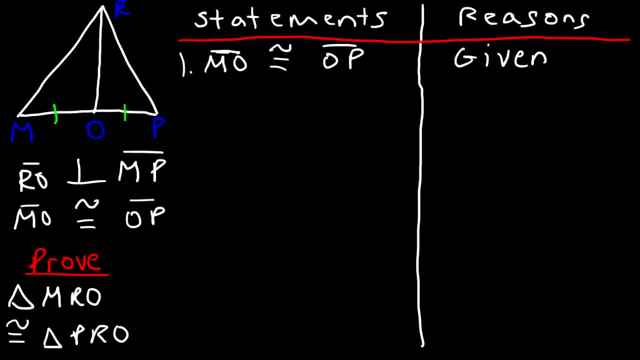 So here's MO and that's congruent to OP. Let's highlight it with tick marks. Now let's move on to statement two, and that is segment RO is perpendicular to segment MP, So that's a given. Now, this is RO and this is MP. 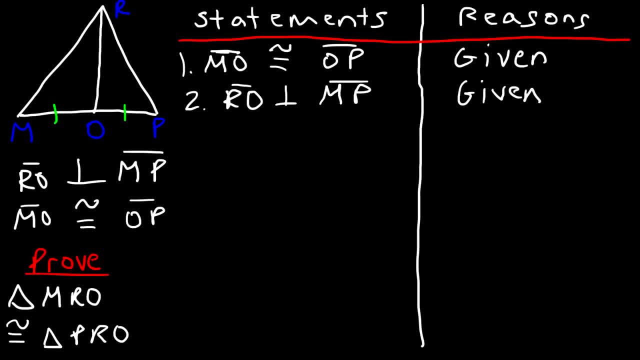 So they're perpendicular. What conclusions can you draw from perpendicular lines? At what angles do perpendicular lines meet? A perpendicular line will always form a 90-degree angle with the line that it intersects with, So The angle between RO and MO is 90.. 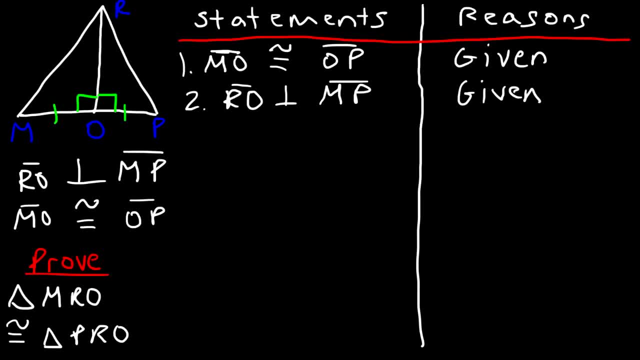 The same is true between RO and OP. Perpendicular lines intersect at right angles. So therefore we could say that Angle MOR is congruent to angle POR And the reason We could say definition of perpendicular lines or simply that perpendicular lines 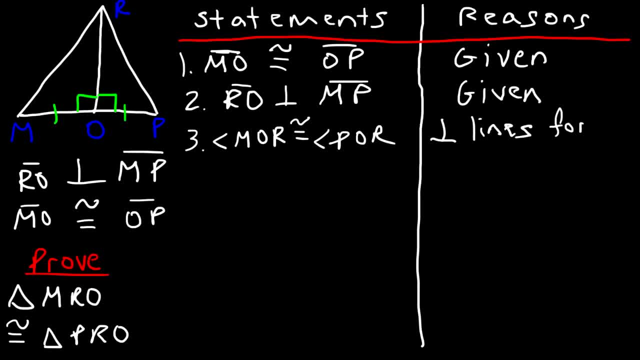 Form: right angles. Now, what else can we say? Now, notice that we do have a common side. So for statement four, we could say that RO is congruent to RO, And we know the reason for that: That's because we have a common side. 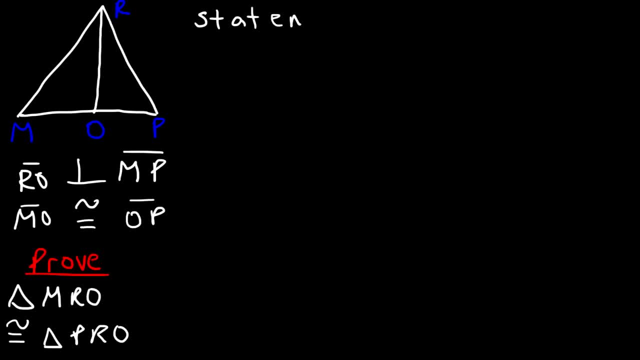 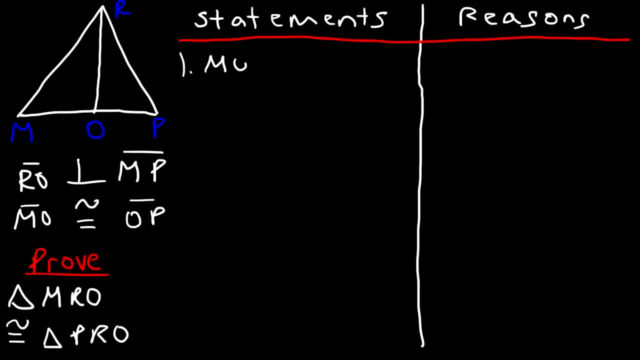 So first let's start with the fact that segment MO is congruent to segment OP And that's given. And just to keep things in perspective, just to make it easier, let's highlight that. So here's MO and that's congruent to OP. 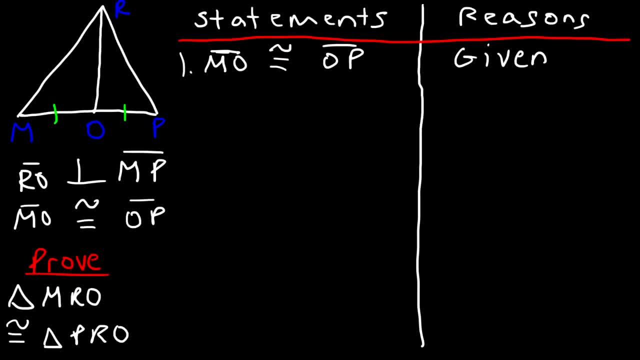 Let's highlight it with tick marks. Let's highlight it with tick marks. Now let's move on to statement 2.. And that is, segment RO is perpendicular to segment MP, to segment MP. So that's a given, So that's a given. 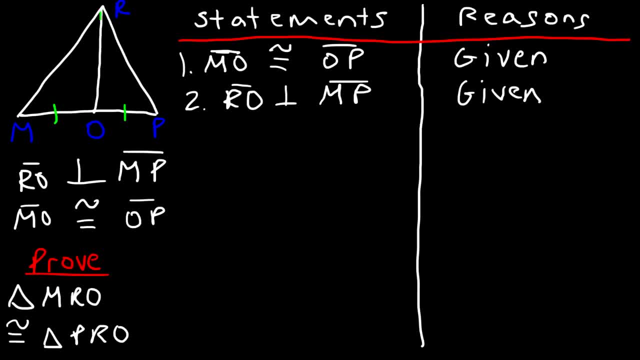 Now, this is RO and this is MP, So they're perpendicular. What conclusions can you draw from perpendicular lines? At what angles do perpendicular lines meet? A perpendicular line will always form a 90 degree angle with the line that it intersects with, So 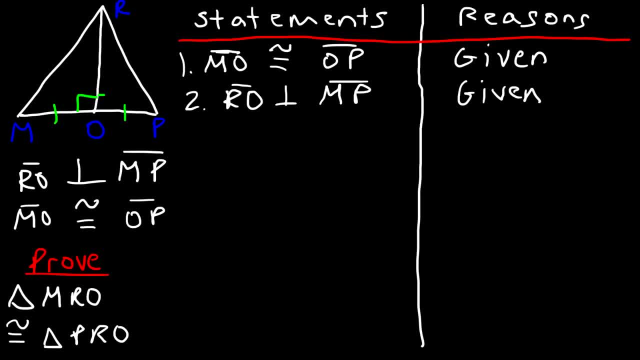 the angle between RO and MO is 90. The same is true between RO and OP. Perpendicular lines intersect at right angles, So therefore we could say that angle MOR is congruent to angle POR And the reason we can say: definition of perpendicular lines. 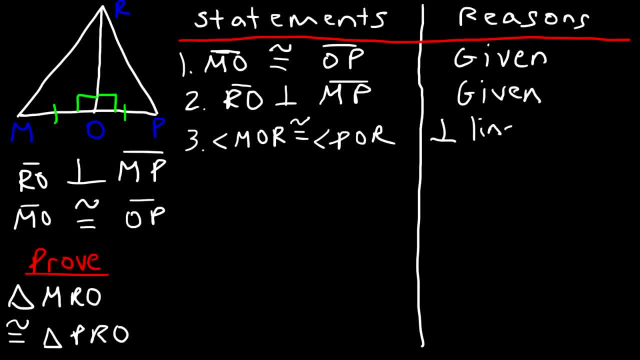 or simply that perpendicular lines form right angles. Now what else can we say? Now, notice that we do have a common side. So for statement 4, we could say that RO is congruent to RO, And we know the reason for that. That is the 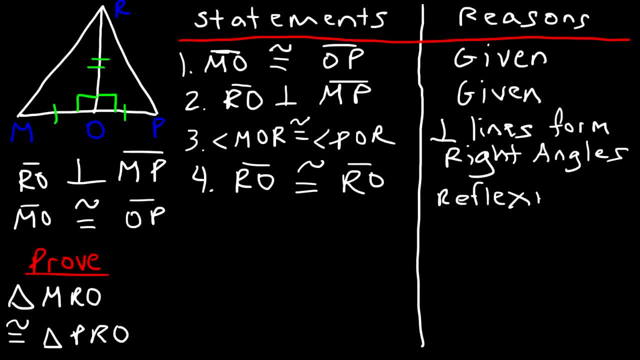 And that is the reflexive property. So now we have a side, we have an angle and another side, So we can make the statement that Triangle MRO is congruent to triangle PRO And this is based on the SAS side angle sign. 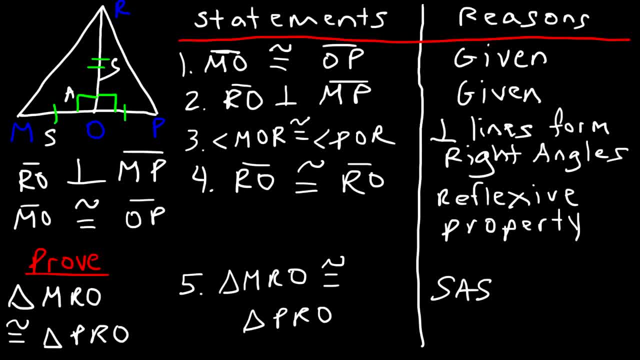 And so we've used, in this example, statement one, which showed that MO is congruent to OP. We use number three- the two angles are congruent- And number four for the common side. So this is based on statements one, three and four. 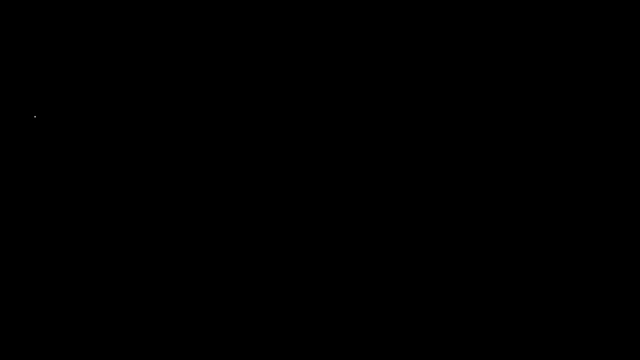 And so that's it. Now let's move on to our next example. So let's say: this is A, B, C, D and E. We're going to call this angle one, angle two, three and four. 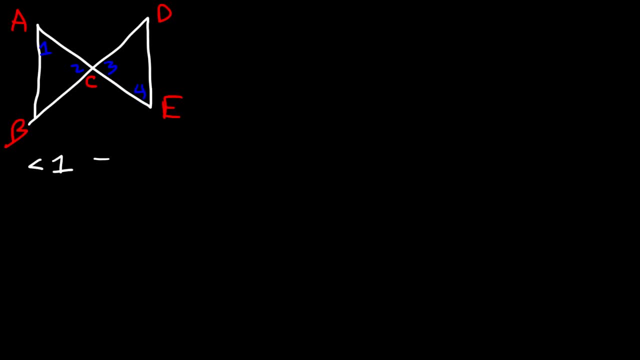 So, given that angle one is congruent to angle four and also that segment AC is congruent to segment C, we're going to call this angle one, angle two, three and four If we go ahead and prove that, go ahead and prove that triangle ABC is congruent to triangle ECD. 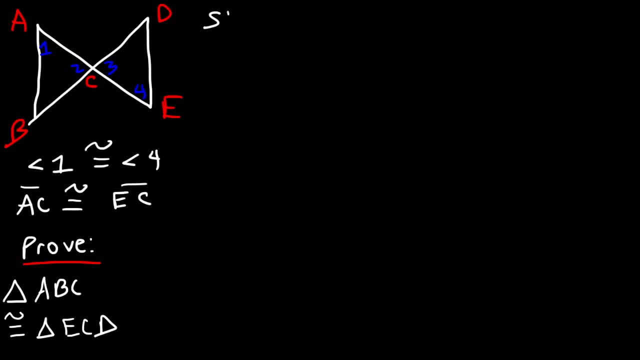 So, once again, pause the video and go ahead and work on this problem. So hopefully by now you're getting the hang of this of how to do these kinds of problems. So I'm going to give you a lot of practice problems. 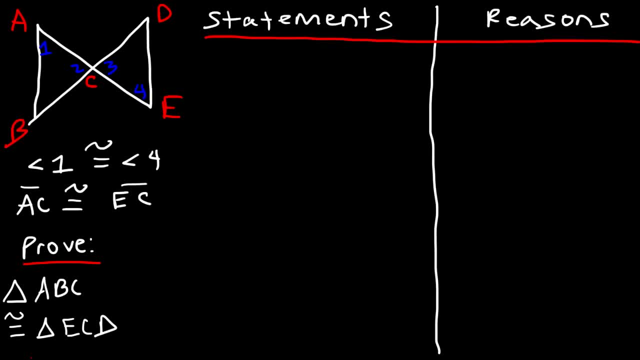 so you can master this topic. So statement one: we can say that angle one is congruent to angle four, And that statement was given to us. So now let's mark it on the diagram. So angle one is congruent to angle four. 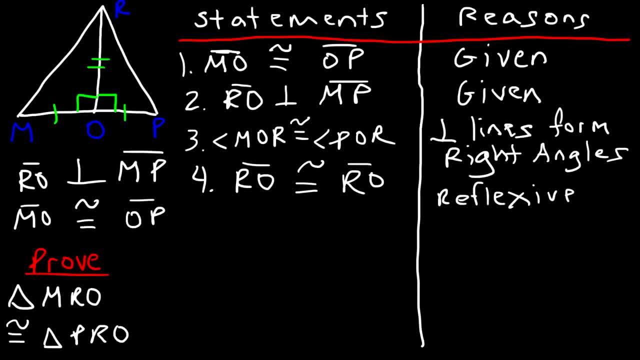 reflexive property. So now we have a side, we have an angle and another side, So we can make the statement that triangle MRO is congruent to triangle PRO, And this is based on the SAS side angle side postulate, And so we've used 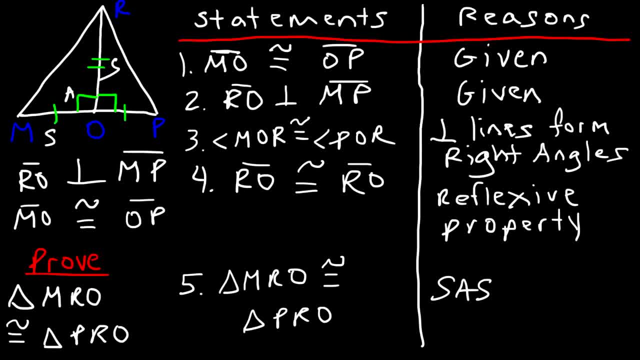 in this example, statement 1 and statement 2, which showed that MO is congruent to OP, We use number 3- the two angles are congruent- and number 4 for the common side. So this is based on statements 1, 3,. 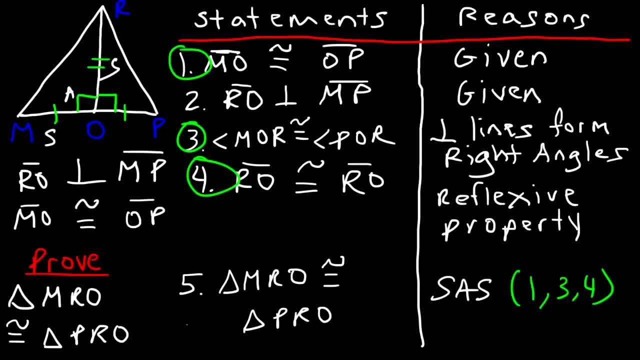 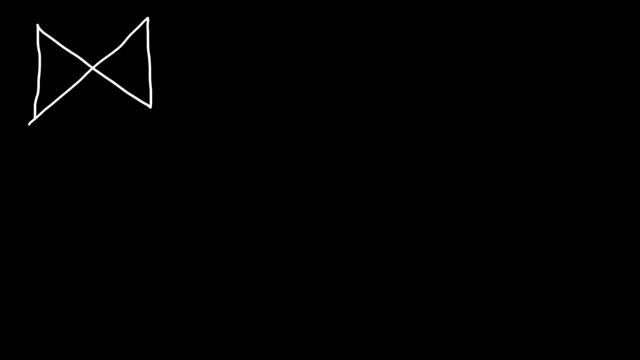 and 4.. And so that's it. Now let's move on to our next example. So this is based on statement 1, so let's say this is A, B, C, D and E. We're going to call this. 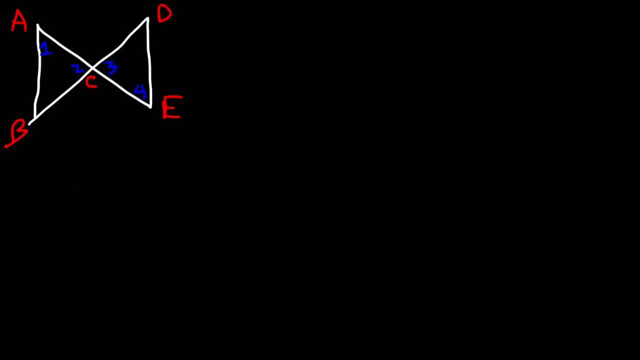 angle 1,, angle 2,, 3, and 4.. So, given that angle 1 is congruent to angle 4 and also that segment AC is congruent to segment EC, prove- go ahead and prove that triangle ABC is congruent to triangle. 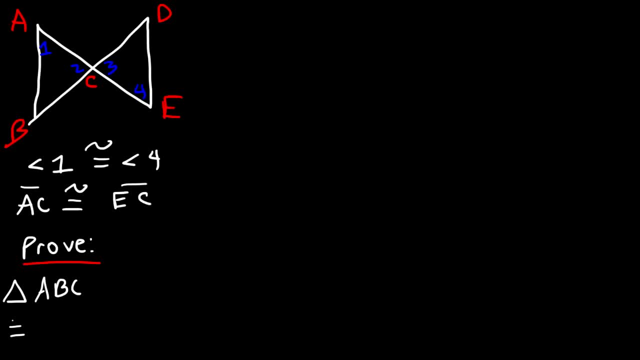 ECD. So, once again, pause the video and go ahead and work on this problem. So hopefully by now you're getting a hang of how to do these kinds of problems. Thank you, Thank you. So I'm going to give you a lot of practice. 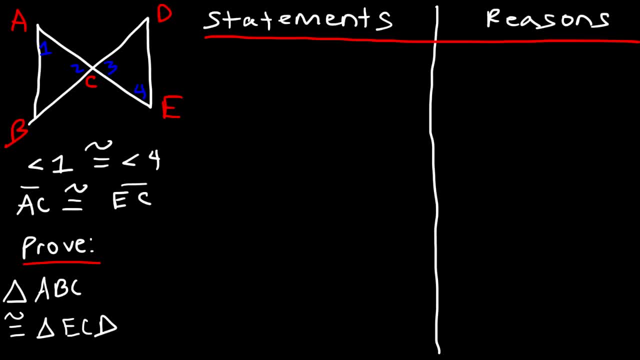 problems so you can master this topic. So statement 1, we can say that angle 1 is congruent to angle 4. And that statement was given to us, So now let's mark it on the diagram. So angle 1 is congruent. 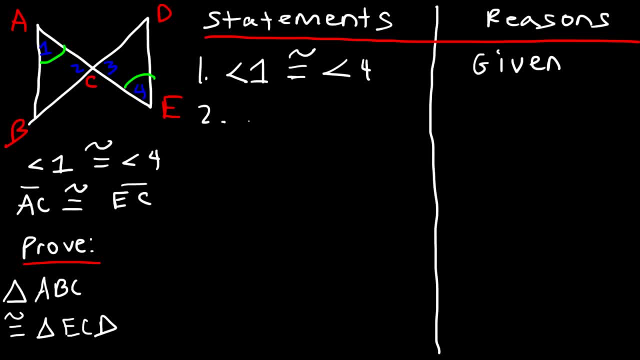 to angle 4.. Now statement 2,: segment AC is congruent to segment EC, And that's given to us as well. So here is segment. let me use a different color. This is segment AC and here is EC. Now, what else can we say? 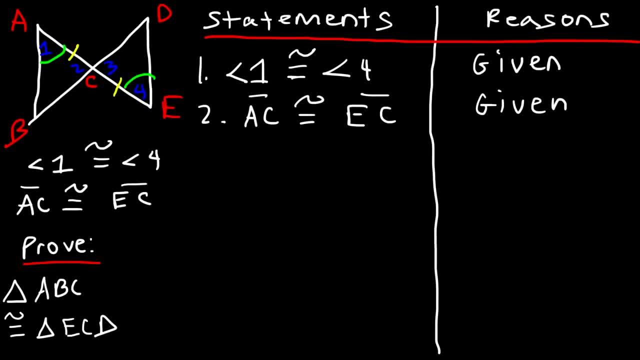 about the two triangles. Now notice that we have vertical angles. Angle 2 is congruent to angle 3.. And why can we say that? Why is angle 2 congruent to angle 3? These two are vertical angles, And remember vertical angles. 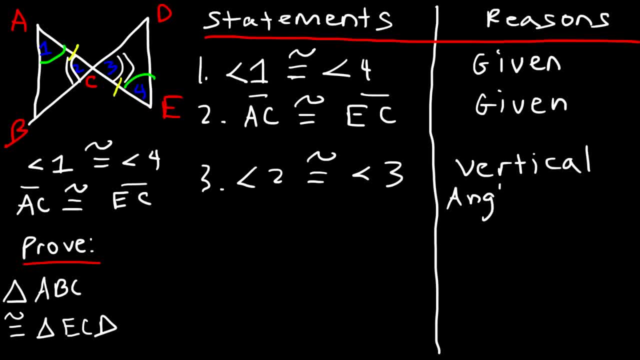 are congruent. So now we have three things: We have an angle, we have a sign- I mean a side by the yellow mark there- and we have another angle. So by the ASA postulate we can say that triangle ABC is congruent. 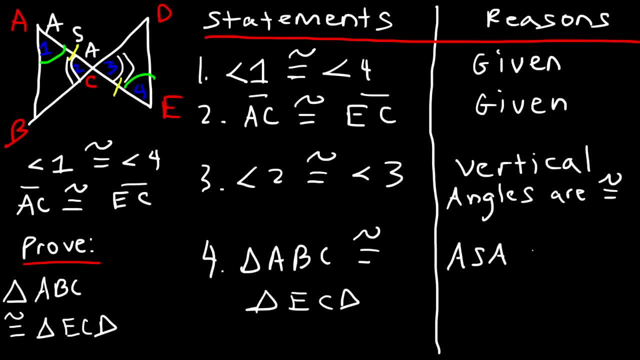 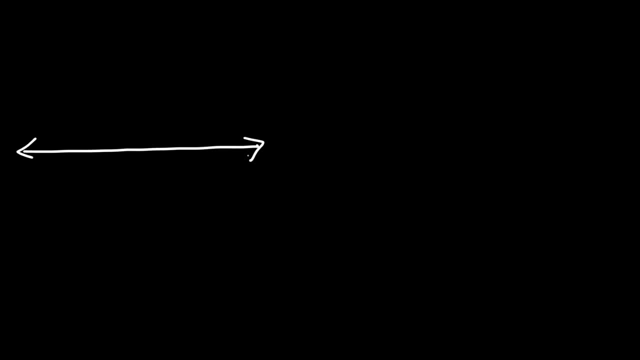 to triangle ECD, And the numbers that we use are basically 1,, 2, and 3.. It's based on statements 1,, 2, 3.. Alright, let's try another example. So let's say this is: 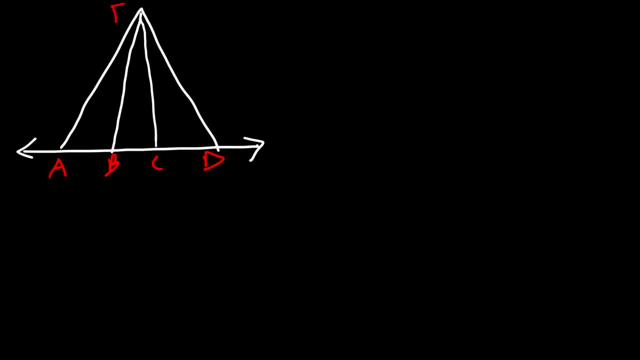 A, B, C, D and E. So we're given that segment AB is congruent to CD And segment AE is congruent to segment DE, And also that angle 1 is congruent to angle 4. And I need to write those angles. 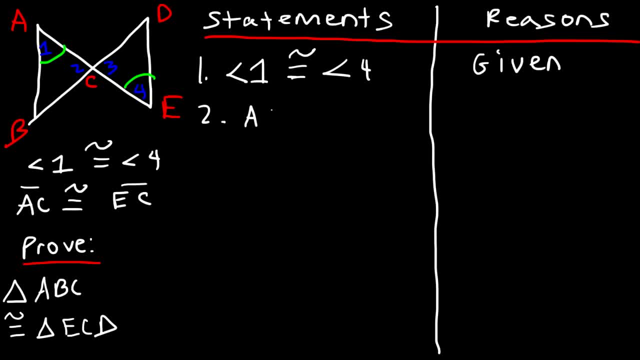 Now statement two. we know that segment AC is congruent to segment EC, And that's given to us as well. So here is segment. I'm going to use a different color. This is segment AC and here is EC. Now what else can we say about the two triangles? 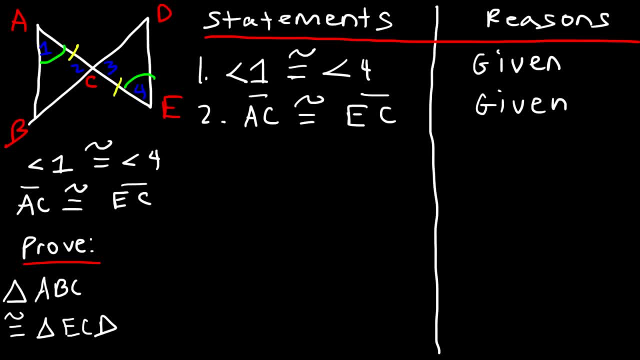 Now notice that we have vertical angles. Angle two is congruent to angle three. And why can we say that? Why is angle two congruent to angle three? These two are vertical angles And remember, vertical angles are congruent. So now we have three things. 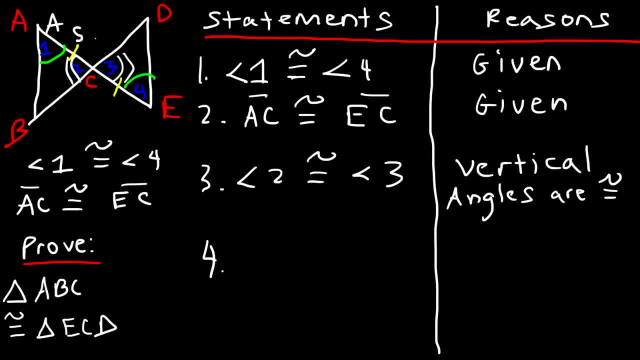 We have an angle, we have a side by the yellow mark there and we have another angle. So by the ASA postulate we can say that triangle ABC is congruent to triangle ECD And the numbers that we use are basically one, two and three. 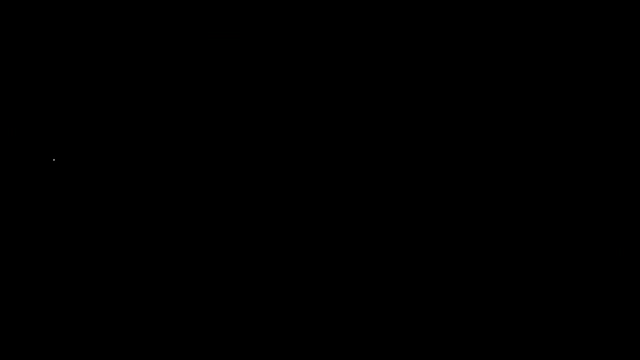 It's based on two Statement's: one, two, three. All right, let's try another example. So let's say this is A, B, C, D and E. So we're given that segment AB is congruent to CD. 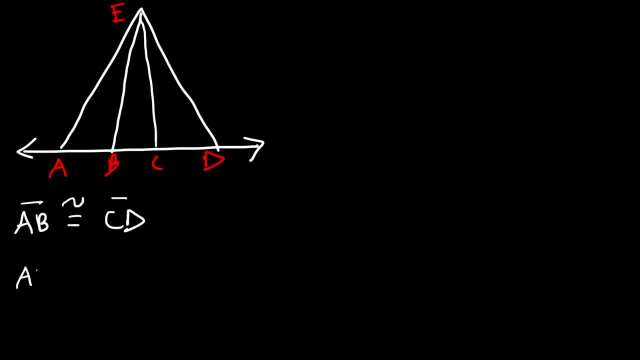 And segment AE is congruent to segment DE, And also that angle one is congruent to angle four, And I need to write those angles. This is angle one, two, three and four, And three is on the inside, All right. 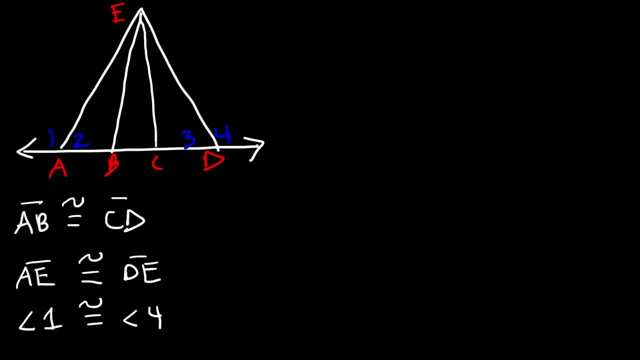 This is angle 1,, 2,, 3, and 4.. And 3 is on the inside. Your task is to prove that triangle is ABE, is congruent to triangle DCE. So go ahead and take a minute and work. 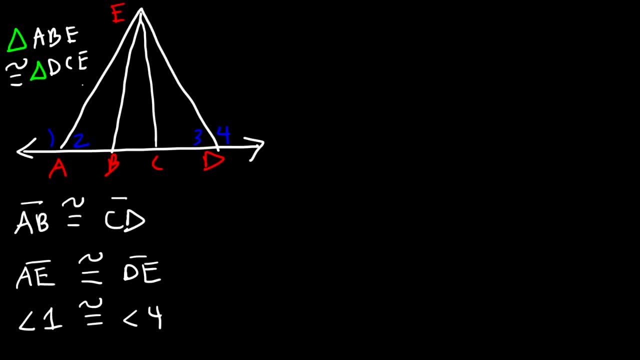 on that example. So how should we begin? Well, let's write the two columns: statements and reasons. So the first statement we're going to say is that AB is congruent to CD, which is given And, as always, we're going to mark this. 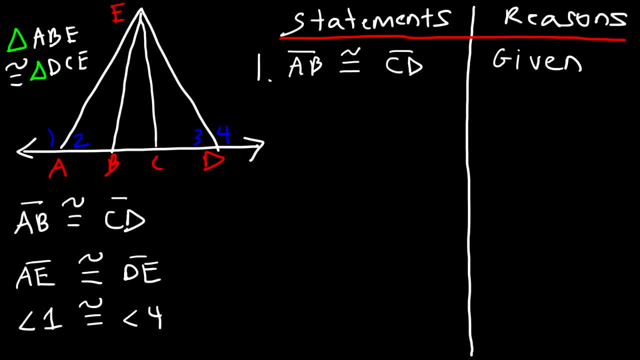 on a graph. So this is AB and here's CD. Now the second statement is that AE is congruent to DE, which is also given, And so this is AE and this is DE. Now we're given that angle 1. 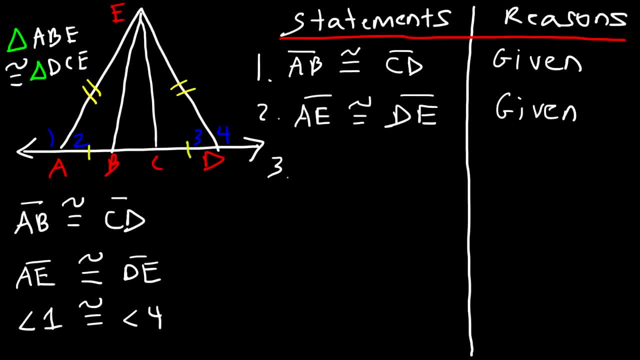 is congruent to angle 4.. So we're going to write that as well. Angle 1 is congruent to angle 4.. So these two are the same. Now, if those two angles are the same, then the angles that are supplementary. 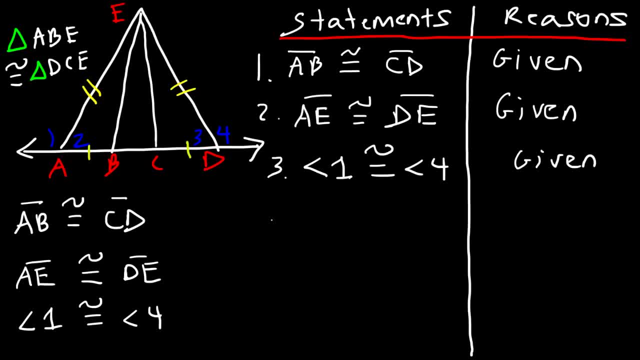 to those angles 2 and 3 are the same as well. So in step 4, we can say that angle 2 is congruent to angle 3. And the reason for that is that supplements of congruent angles are congruent. 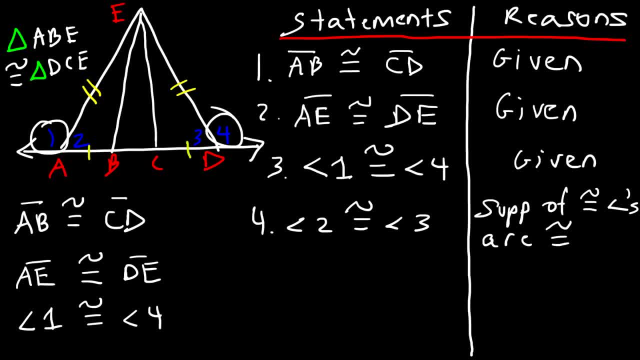 So let's say, if angle 1 was 120, angle 4 has to be 120. That means number 2 has to be 60.. 60 plus 120 is 180.. So 3 is 60, which means 2 equals 3.. 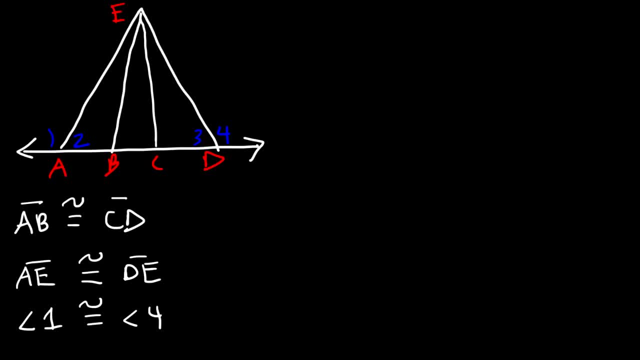 Your task is to prove that triangle ABE is congruent to triangle DCE. So go ahead and take a minute and work on that example. So how should we begin? Well, let's write the two columns: Statements and reasons. So the first statement we're going to say is that AB is congruent to CD. 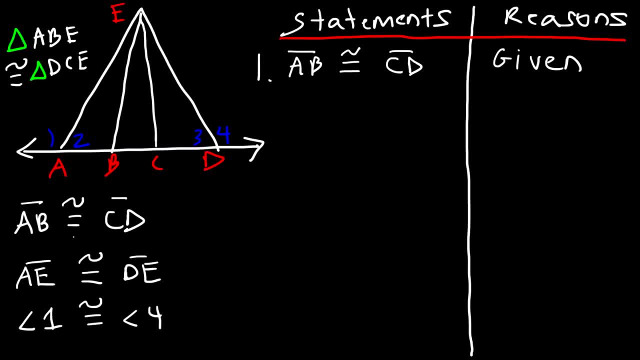 which is given, And, as always, we're going to mark this on the graph. So this is AB and here's CD. Now the second statement is that AE is congruent to DE, which is also given, And so this is AE and this is DE. 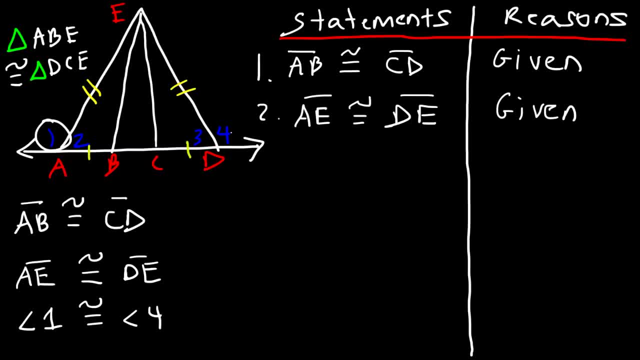 Now we're given that angle one is congruent to angle four, So we're going to write that as well: Angle one is congruent to angle four, So these two are the same. Now, if those two angles are the same, 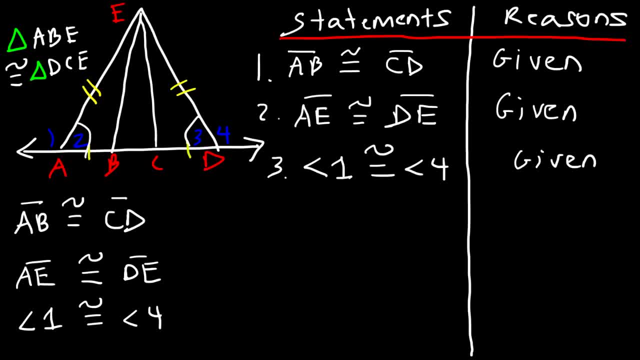 then the angles that are supplementary to those angles, two and three are the same as well. So in step four we could say that angle two is congruent to angle three, And the reason for that is that supplements of congruent angles are congruent. 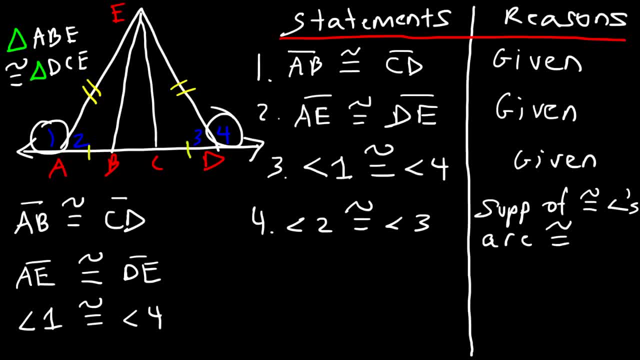 So let's say, if angle one was 120, angle four has to be 120. That means number two has to be 60,. 60 plus 120 is 180.. So three is 60, which means two equals three. Okay. 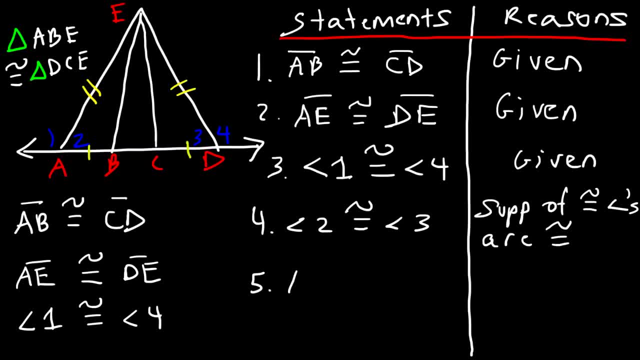 Now step 5.. We can make the final statement that triangle ABE is congruent to triangle DCE. Now what postulate can we use to show that those two triangles are congruent? So let's see We have, let's mark, that these two are congruent. 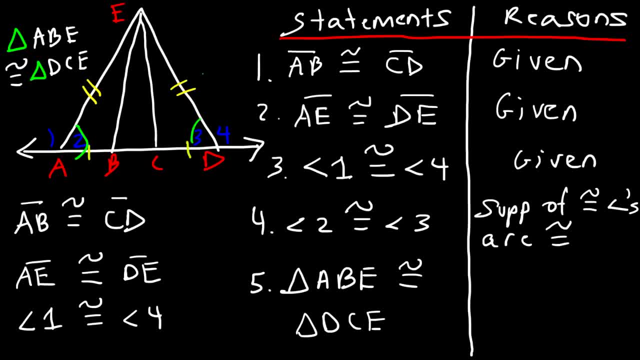 Angles 2 and 3. So we have a side, an angle and a side. So hopefully you see it, You can also see on this side too, Side, angle side. So it's the SAS postulate And we've used. 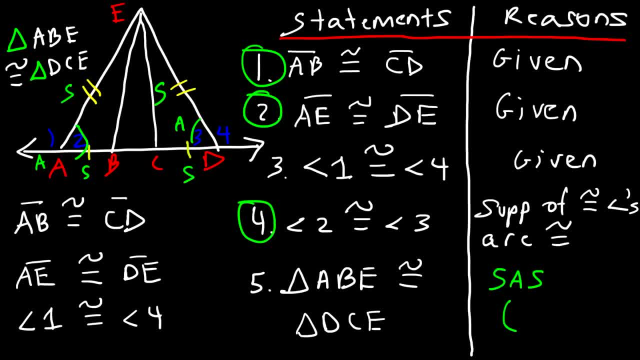 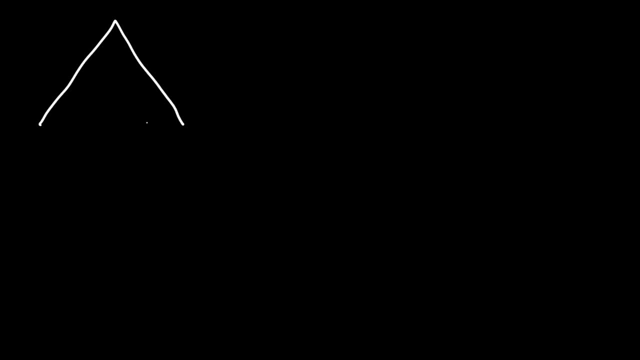 statements 1,, 2, and 4 to accomplish the congruence of these two triangles. So it's 1, 2, and 4.. And that's it for this problem. Here's another one that we can work on. 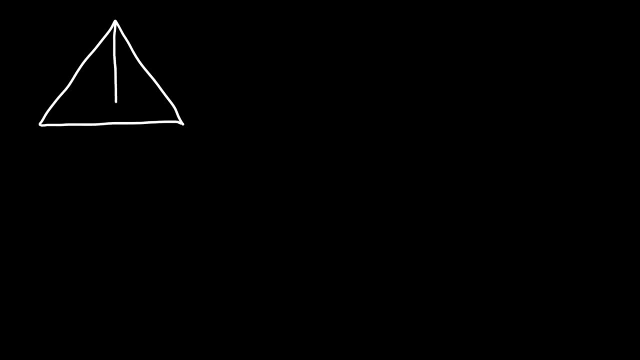 Similar to the first two, but with a few differences. So let's call this T Q R and S, And we're given that angle T Q R is congruent to angle T S R, And we're also given 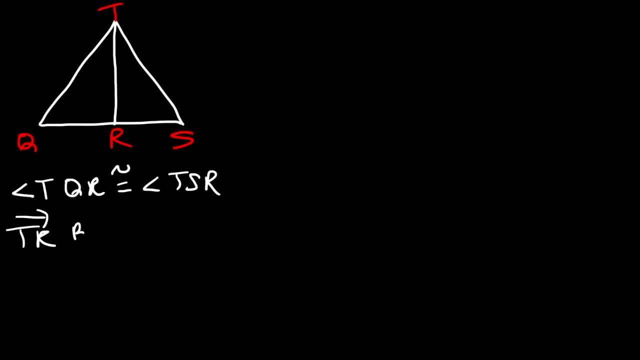 that T R bisects angle Q T S. So your task is to prove that triangle Q T R is congruent to triangle S T R. So go ahead and work on it. So number one: 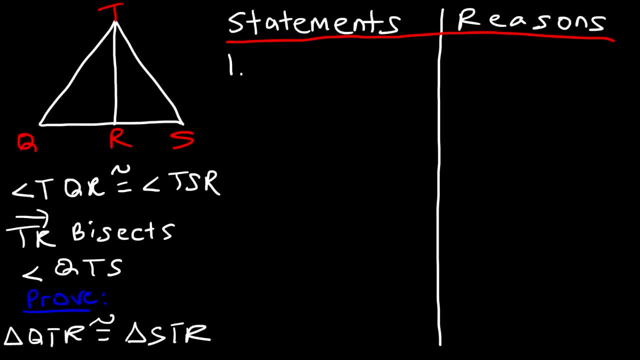 The given T Q R is congruent to T S R. So T Q R, we could describe it as angle Q, And T S R we could say is just angle S, Because angle Q can only 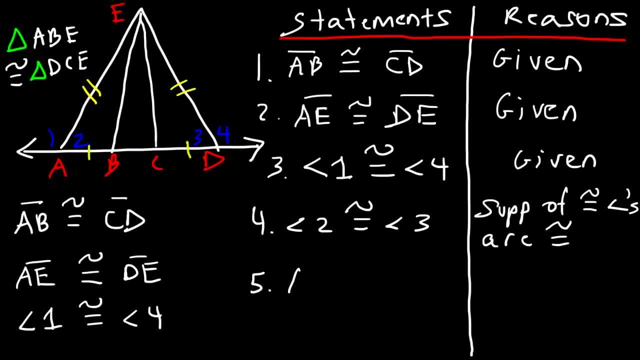 Now step five. we can make the final statement that triangle ABE is congruent to triangle DCE. Now what postulate can we use to show that those two triangles are congruent? So let's see, We have- Let's mark that these two are congruent- angles two and three. 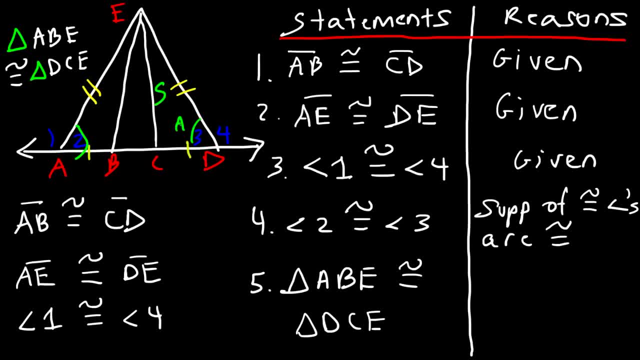 So we have a side, an angle and a side. So hopefully you see it, You can also see on this side too, Side angle side. So it's the SAS postulate And we've used statements one, two and four. 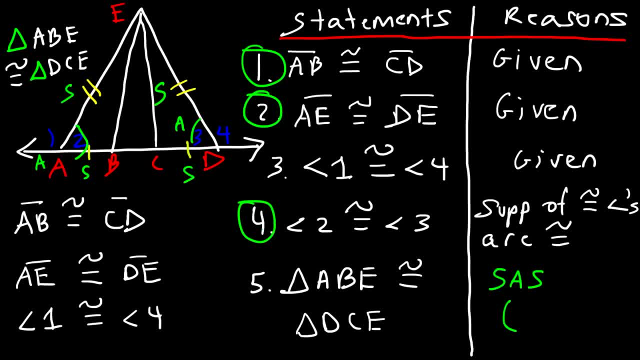 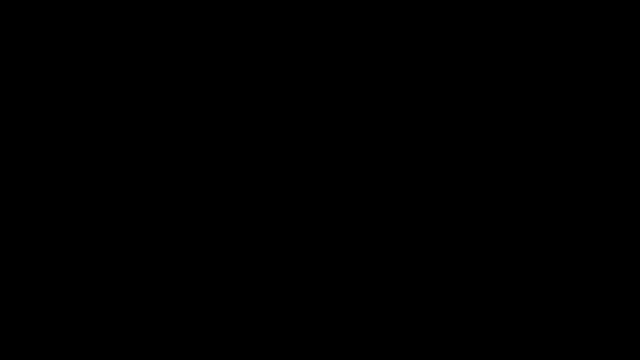 to accomplish the congruence of these two triangles. So it's one, two and four, And that's it for this problem. Here's another one that we can work on, Similar to the first two, but with a few differences. 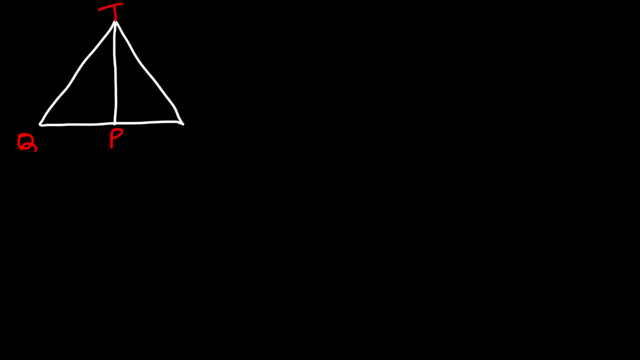 So let's call this T, Q, R and S, And we're given that angle T Q R is congruent to angle T S R, And we're also given that T R bisects angle Q T S. 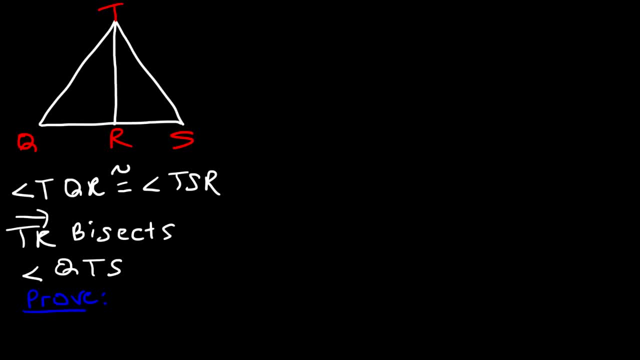 So your task is to prove that triangle Q T R is congruent to triangle S T R. So go ahead and work on it. So, number one, the given T Q R is congruent to T S R. 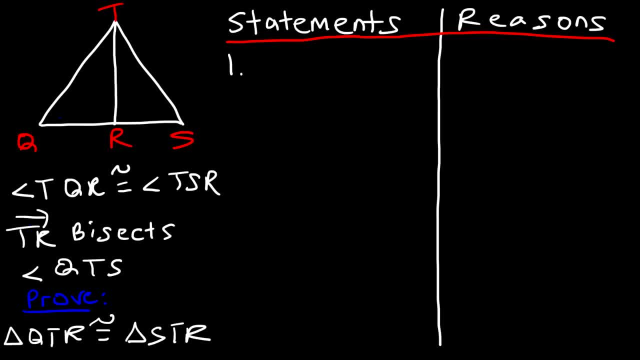 So T Q R- we could describe it as angle Q, And T S R, we could say is just angle S, Because angle Q can only correspond to this angle. So I'm going to say angle Q is congruent to angle S. 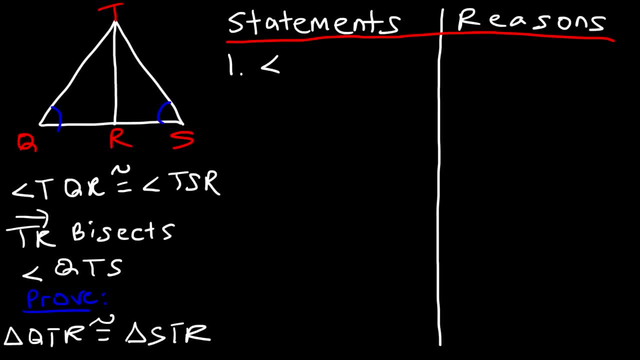 correspond to this angle. So I'm going to say angle Q is congruent to angle S. Let's write it. And the reason is that it's given. Now number two: We know that ray T R bisects angle Q, T, S. 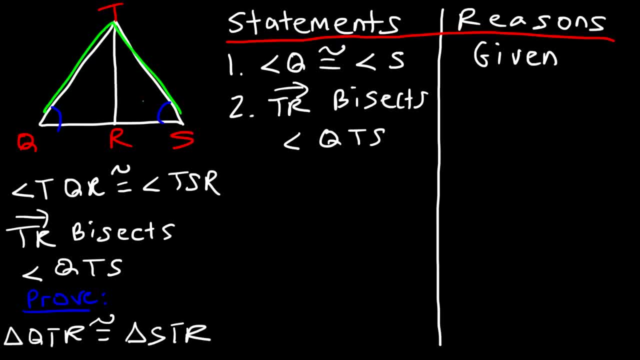 So this is Q T X And this is ray T R. It bisects it or splits it into two congruent angles, Which means that these two angles are congruent. Let's put the reason for statement two as given. 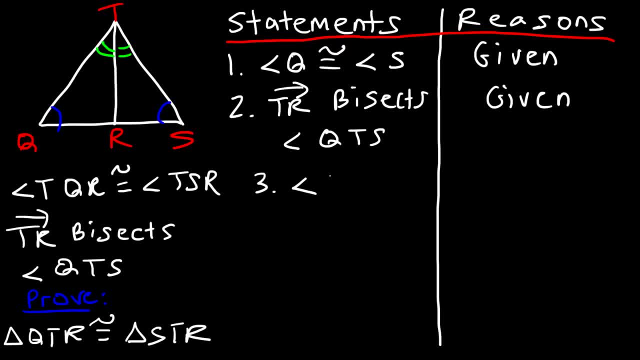 And now statement three. We could say that angle Q T R is congruent to angle S T R. Now the reason for this, that we can write, is based on the definition of an angle bisector. This is an angle bisector. Angle bisectors are: 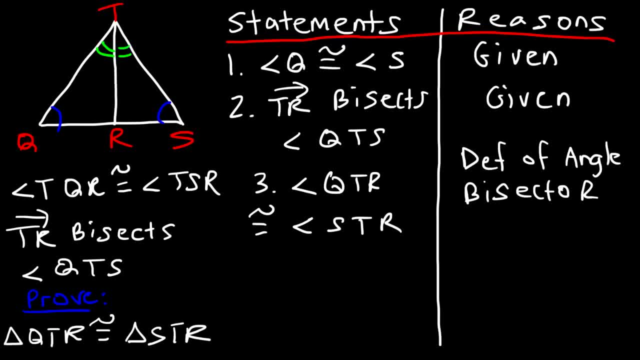 rays And they split an angle into two congruent angles. Now we do have a common side, So every time you have a common side, you can use the reflexive property. So we're going to state that T? R is congruent to itself. T R. 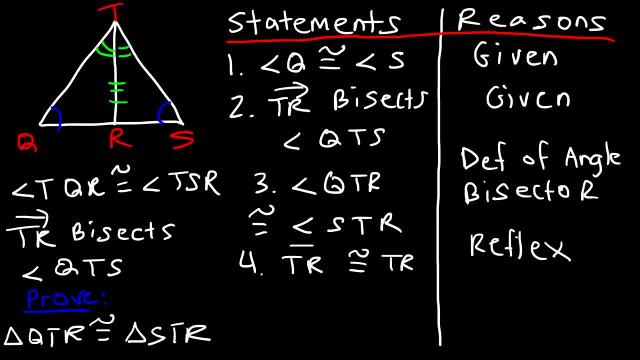 And that's the reflexive property. Now, finally, we can make the fifth statement that triangle Q T R is congruent to triangle S T R. And what postulate can we use to say this? So here we have an angle, another angle. 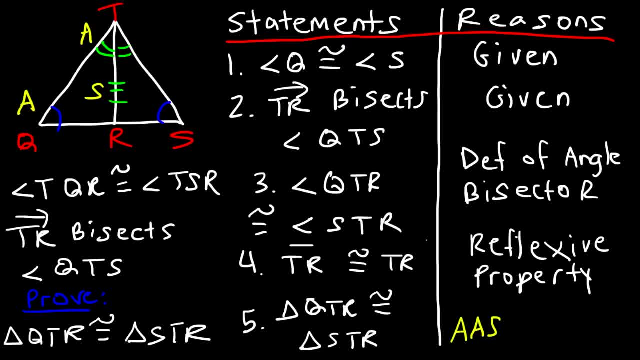 and a side. So this is the A A S postulate And we use number one to prove that angle Q is equal to angle S And number two- that just helps us to establish number three, which we did use, that That's the second angle. 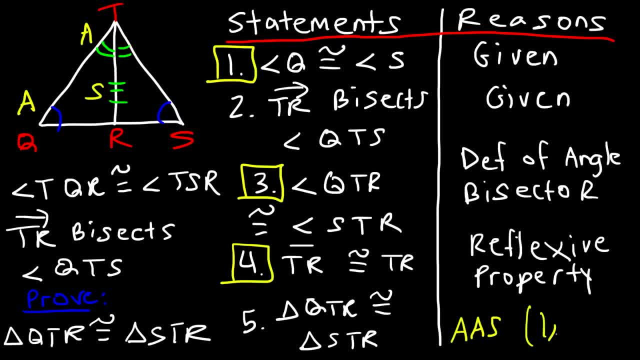 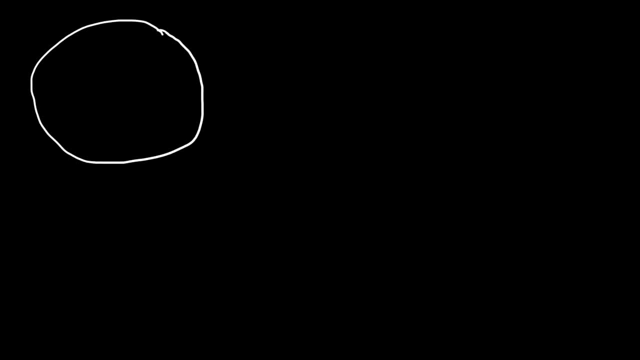 And for the side that's number four. So it's based on statements one, three and four, And that's how you can prove the two triangles using the A, A, S postulate Angle angle side. Now let's move on to our next problem. 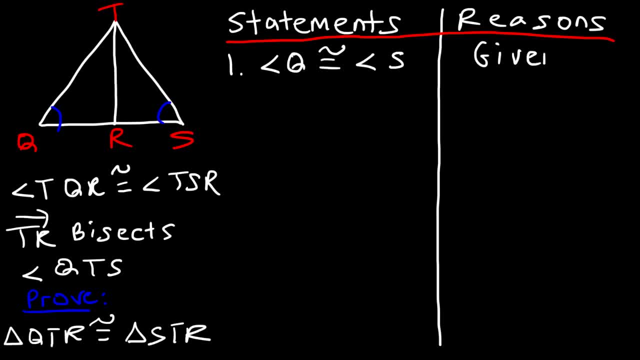 Let's write it, And the reason is that it's given Now number two: we know that ray T R bisects angle Q T S, So this is Q T X And this is ray T R. 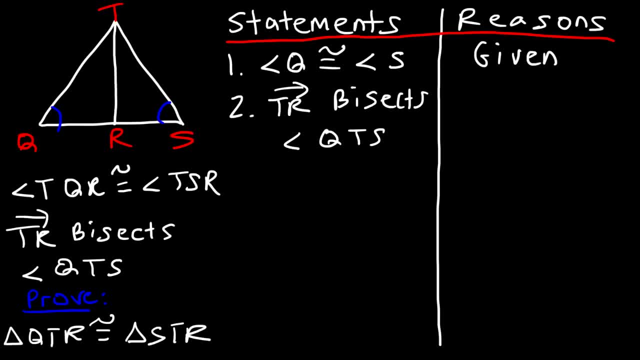 It bisects it or splits it into two congruent angles, Which means that these two angles are congruent. But let's put the reason for statement two is given, And now statement three. we could say that angle Q T R is congruent to angle S T R. 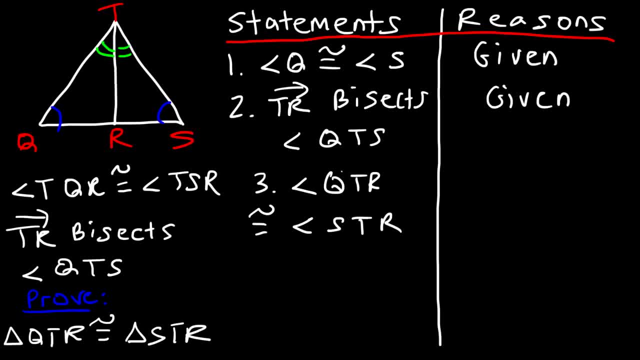 Now, the reason for this is that Now, the reason for this that we can write is based on the definition of an angle bisector. This is an angle bisector. Angle bisectors are rays And they split an angle into two congruent angles. 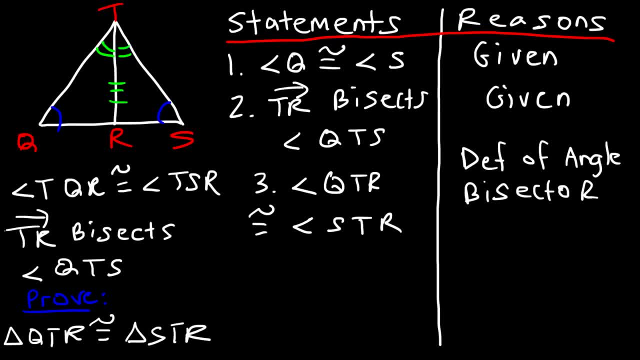 Now we do have a common side. So every time you have a common side, you can use the reflexive property. So we're going to state that T? R is congruent to itself. T? R And that's the reflexive property. 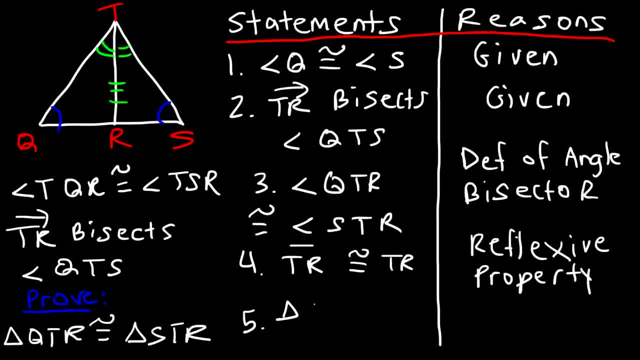 Now, finally, we can make the fifth statement That triangle Q T R is congruent to triangle S T R. And what postulate can we use to say this? So here we have an angle, Another angle and a side. 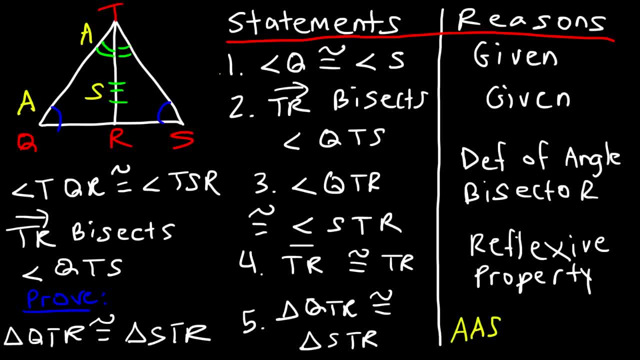 So this is the AAS postulate And we use number one to prove that angle Q is equal to angle S, And number two- that just helps us to establish number three, which we did use- that That's the second angle And for the side, that's number four. 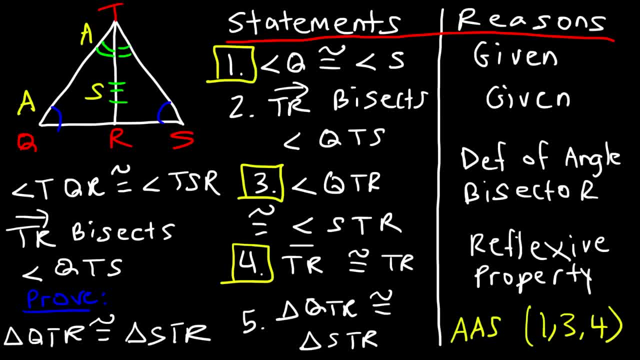 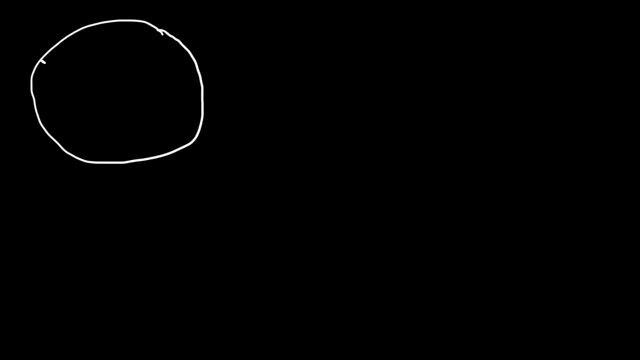 So it's based on statements one, three and four, And that's how you can prove the two triangles using the AAS postulate Angle angle side. Now let's move on to our next problem. So let's call this A, B, C, D and E. 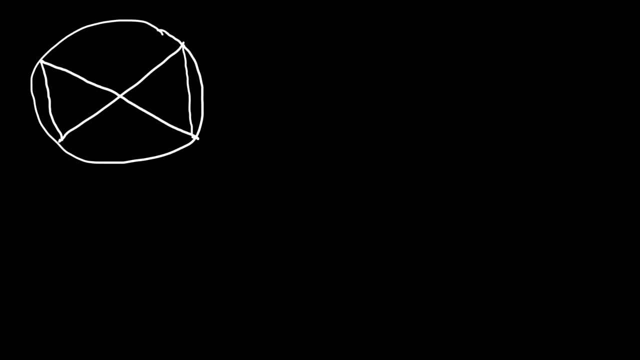 So let's call this A, B, C, D and E, And you're given that C is the midpoint of two segments: C is the midpoint of A- E and it's the midpoint of B- D. So, with this information, 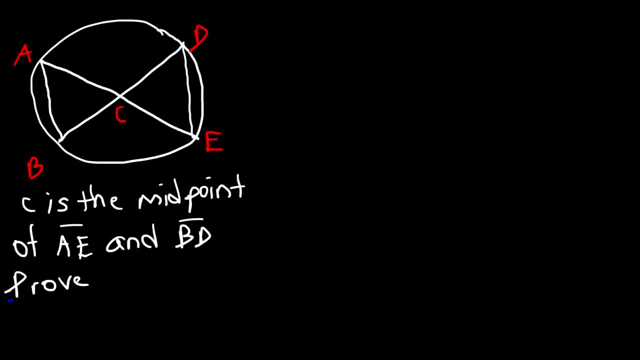 go ahead and prove that triangles A, B, C is congruent to triangle E D C. So how can we prove that triangle A, B, C is congruent to triangle E D C? What would you say? So let's start with the given. 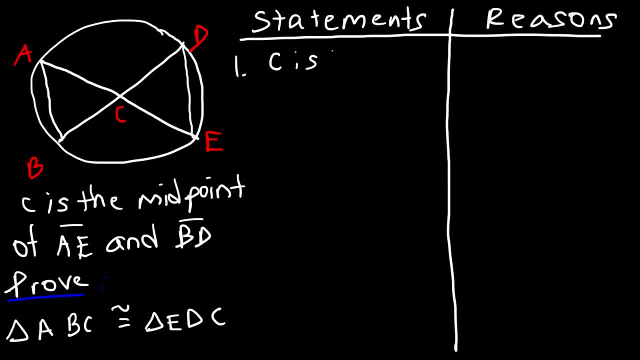 So we're given that C is the midpoint of A- E and B- D. So that's a given. Now number two, because C is the midpoint of A- E. that means that A- E is bisected into two congruent segments. 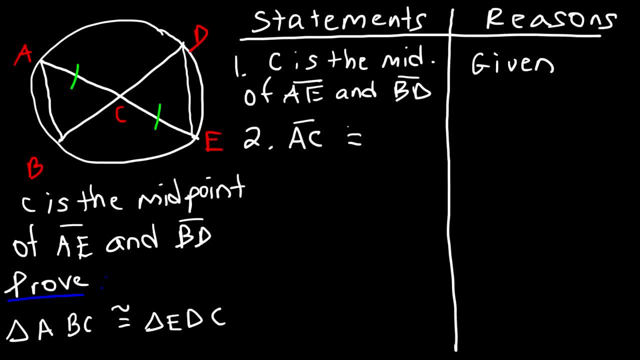 So we could say that A- C is congruent to E- C, And the reason is definition of a midpoint. Now, number three: we could say that B? C is congruent to C- D, Because C is still the midpoint of B? D. 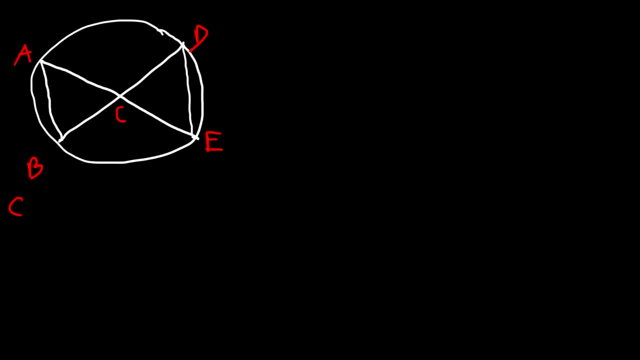 And you're given that C is the midpoint, The midpoint of two segments: C is the midpoint of A- E and it's the midpoint of B- D. So, with this information, go ahead and prove that triangles A, B, C, D and E are congruent. 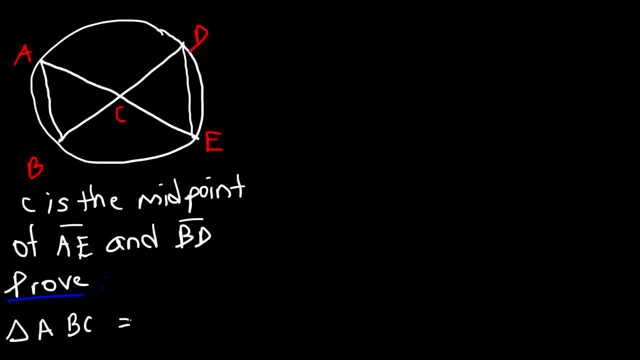 A, B, C is congruent to triangle E D C. So how can we prove that triangle A, B, C is congruent to triangle E D C? What would you say? So let's start with the given. 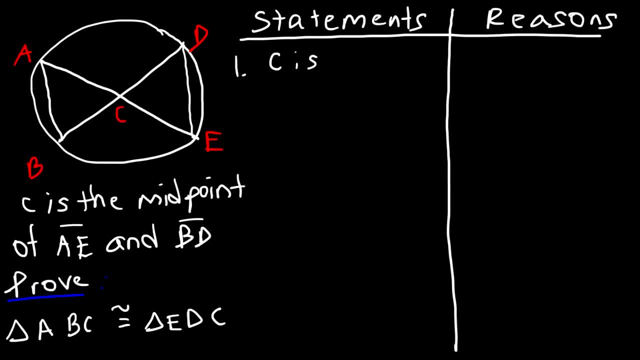 So we're given that C is the midpoint of A- E and B- D. So that's a given. Now number two, because C is the midpoint of A- E. that means that A- E is bisected into two congruent segments. 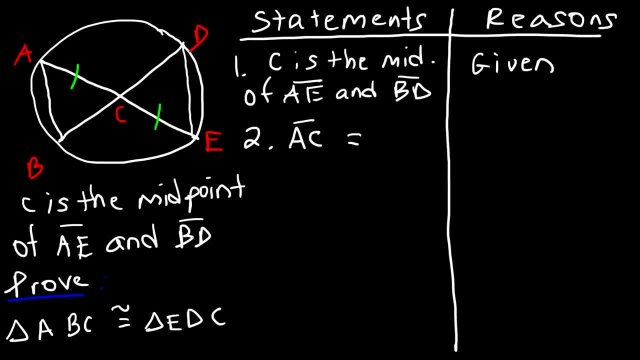 So we could say that A- C is congruent to E- C, And the reason is definition of a midpoint. Now, number three: we could say that B? C is congruent to C- D, because C is still the midpoint of B? D. 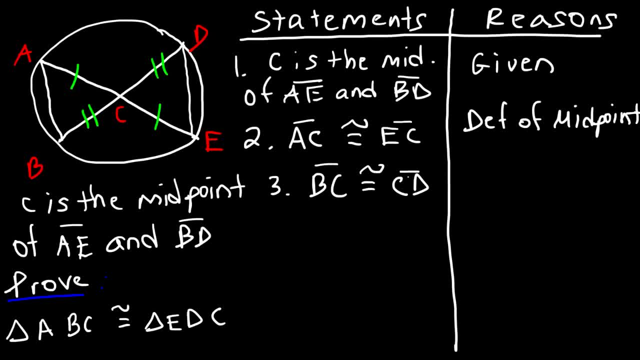 And the reason for that is the same Definition of a midpoint. Now, what else can we say? Another statement that we can make is that angle A, C, B is congruent to angle E, C, D. Now I want to mention that A corresponds to E, not D in this case. 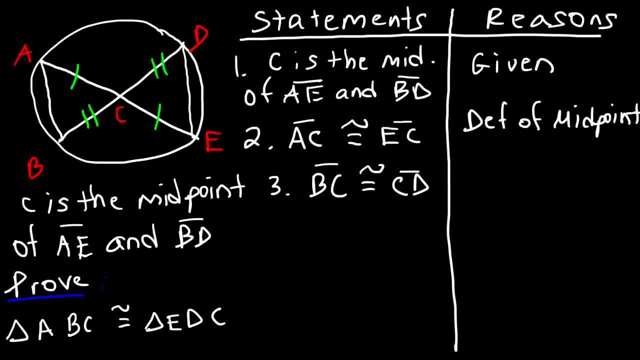 And the reason for that is the same Definition of a midpoint. Now, what else can we say? Another statement that we can make is that angle A C B is congruent to angle E C D. Now, I want to mention that. 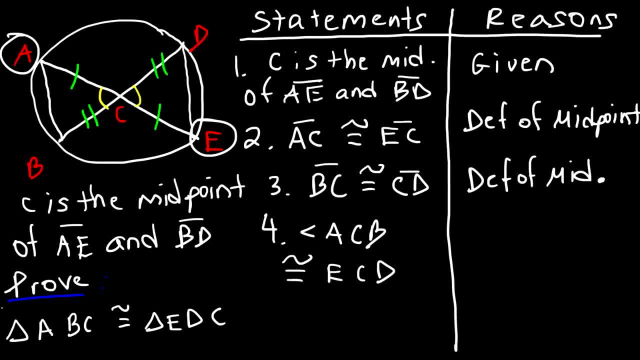 A corresponds to E, not D in this case, Because A is congruent to E, Because look at the angle, or rather the side that angle A is across. Angle A is across the side with two marks And angle E is across the side with two marks. 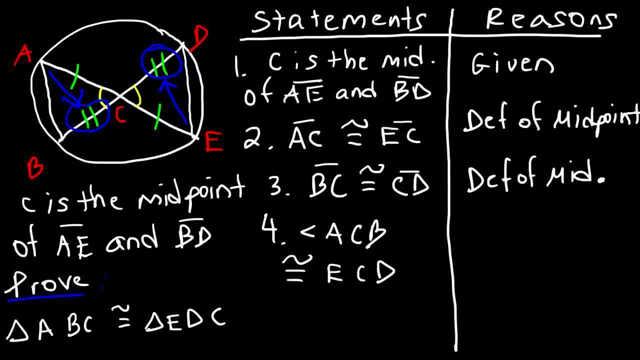 So if these two sides are the same, the angles that are opposite to them should be the same. So that's how we know to match A with E and B with D. So those two angles are congruent. The vertical angles are congruent. 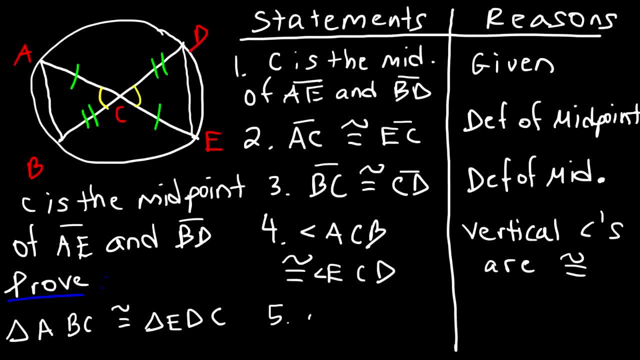 So now we have enough information to prove that triangle A, B, C is congruent to triangle E, D, C. So we have a side, an angle and a side. So using the SAS, we can find out that triangle A is congruent. 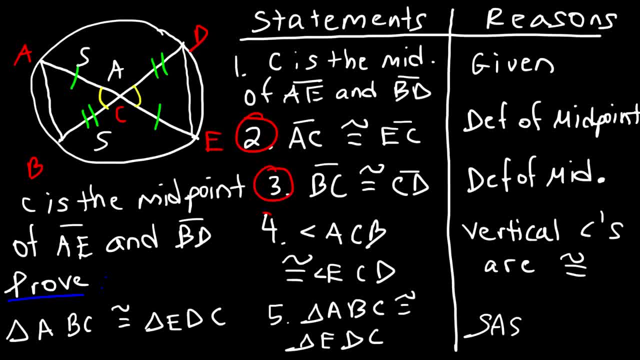 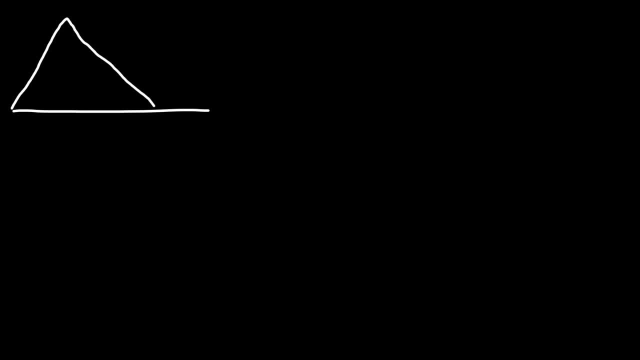 to triangle C. So we've used statement 2,, 3, and 4 to prove that these two triangles are true. So let's write that here And that's it for this problem. So let's say that this is A. 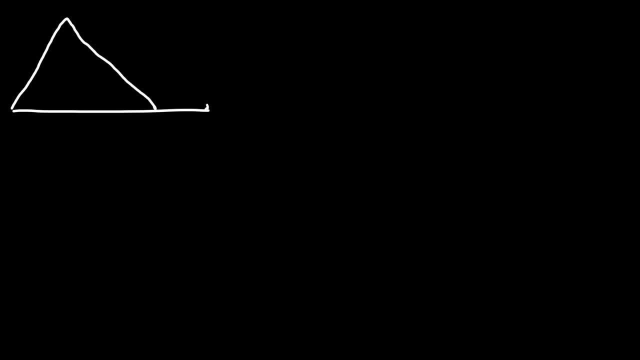 B, C And this is going to be D, E, F And we're given that A- D is congruent to C- F, A- D is congruent to C- F And also that C- B is congruent. 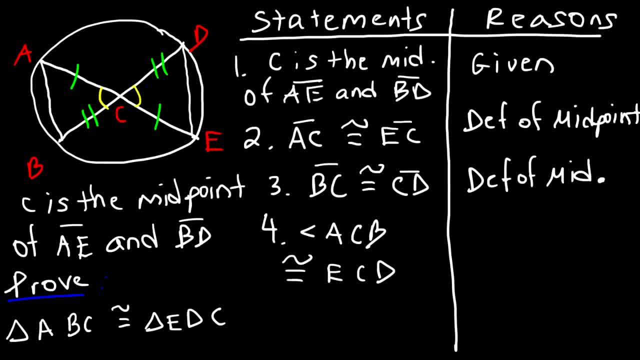 Because look at the angle, or rather the side, that angle A is across. Angle A is across the side with two marks, And angle E is across the side with two marks. So if these two sides are the same, the angles that are opposite to them should be the same. 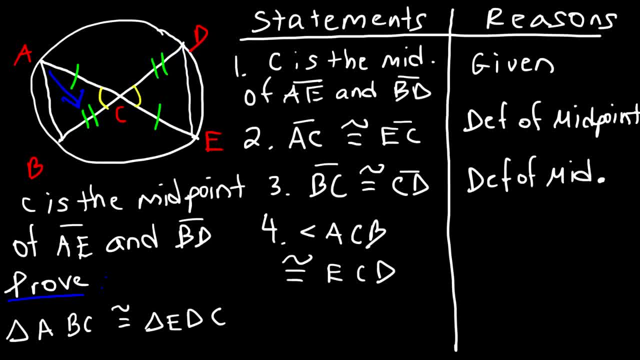 So that's how we know to match A with E and B with D. So those two angles are congruent because the vertical angles are congruent. So now we have enough information to prove that triangle ABC is congruent to triangle EDC. So we have a side, an angle and a side. 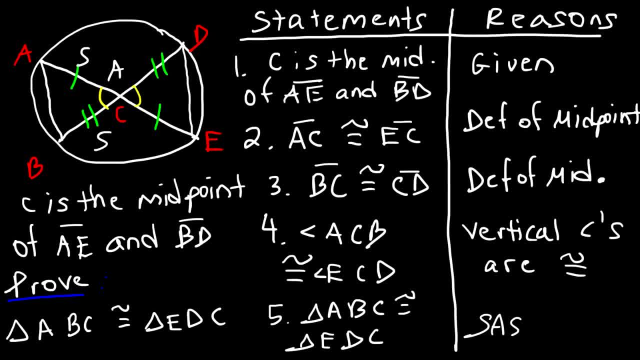 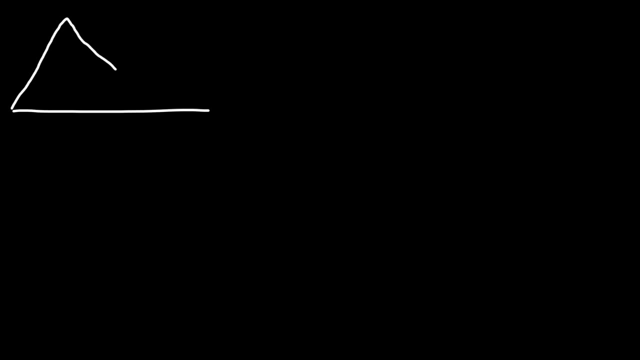 So using the SAS postulate. So we've used statement two, three and four to prove that these two triangles are true. So let's write that here And that's it for this problem. So let's say that this is A, B, C. 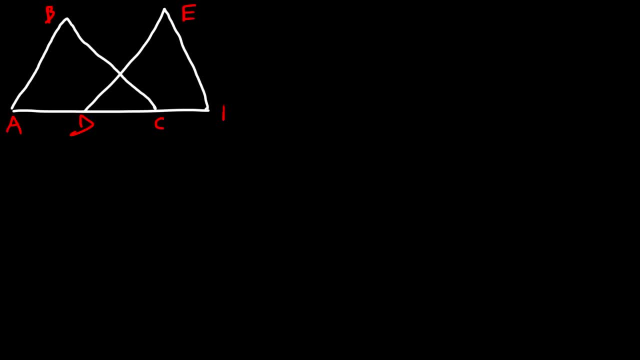 And this is going to be D, E, F, And we're given that A- D is congruent to C- F And also that C- B is congruent to D- E And A- B is congruent to E- F. 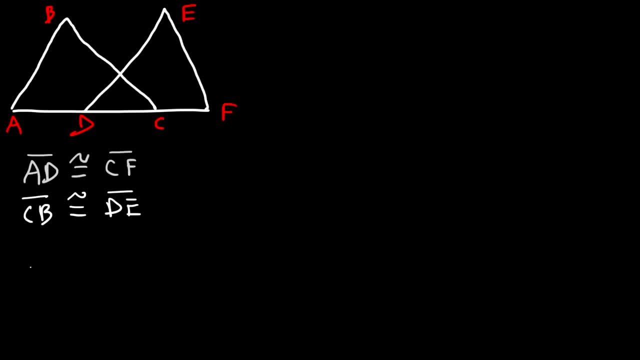 to D, E And A, B is congruent to E, F. Your task is to prove that the two triangles are congruent. So we're going to try to prove that triangle ABC is congruent to triangle F, E, D. 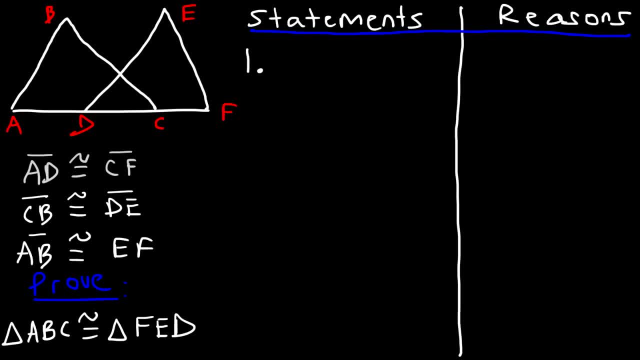 So let's start with the fact that A- D is congruent to C- F, And that's given. And number 2, C- B is congruent to D- E, So that's given as well. And 3,. 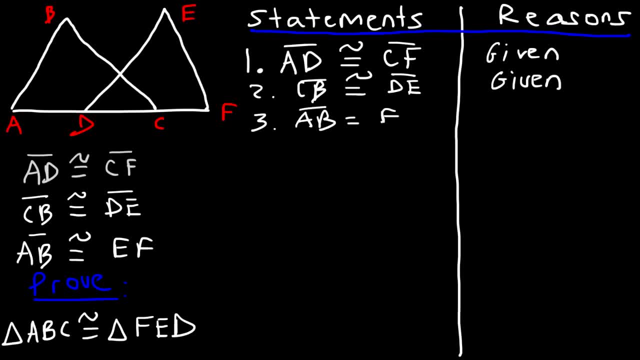 A- B is congruent to E- F. Now the reason why I wanted to write all of that at the beginning is to make some more space. So we know that A- D is congruent to C- F. Now it might be helpful. 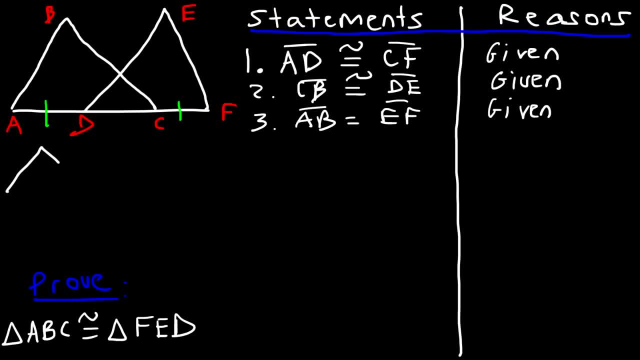 to draw two separate triangles, So this is going to be triangle ABC And that's triangle F E D. Let me use a different color for that. Now, based on statement 2, C B is congruent to D E. 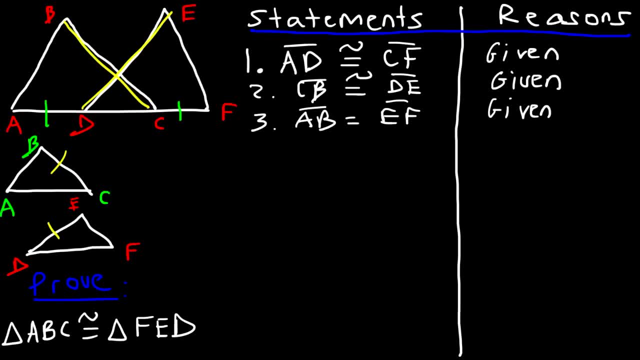 So here's C B and here's D E. Those two sides are congruent And A- B is congruent to E F. So this is AB and this is E F. So if we can prove that AC is congruent to DF, 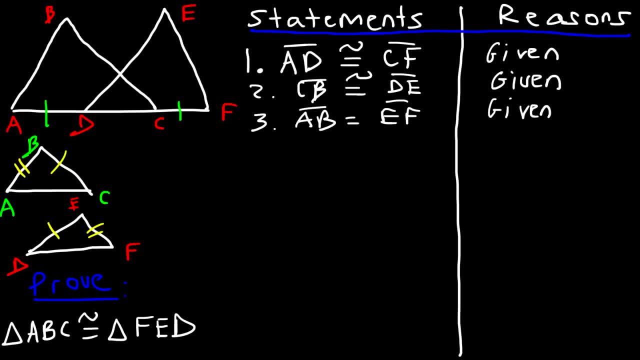 then we can prove that the two triangles are congruent using the SSS postulate. So how can we prove that these two segments are congruent? What can we do So notice that we have an overlapping segment DC, So that implies we need to use segment addition. 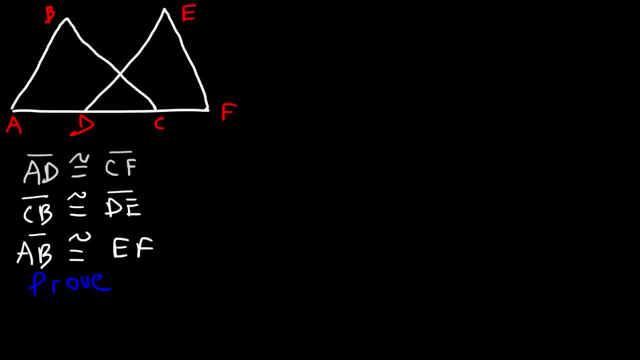 Your task is to prove that the two triangles are congruent. So we're going to try to prove that triangle ABC is congruent to triangle F, E, D. So let's start with the fact that A- D is congruent to C- F. 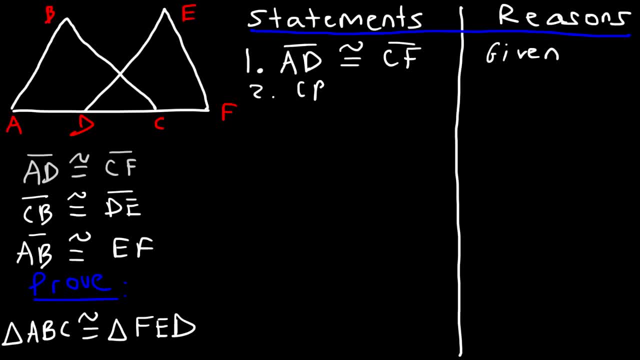 And that's given. And number two C- B is congruent to D- E, So that's given as well. And three A B is congruent to C- F And number three A- B is congruent to E- F. 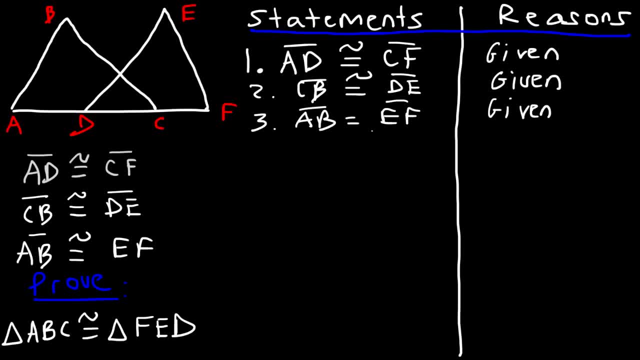 Now, the reason why I wanted to write all of that at the beginning is to make some more space. So we know that A- D is congruent to C, F. Now it might be helpful to draw two separate triangles. So this is going to be triangle. 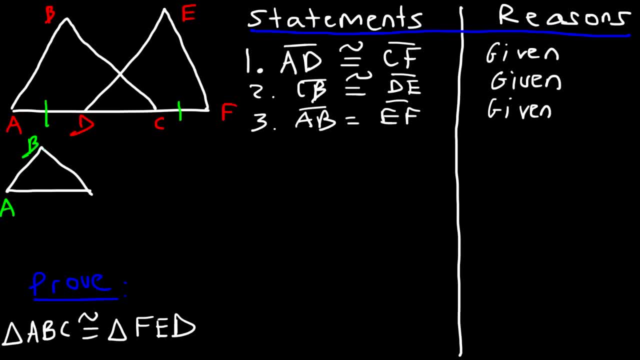 ABC A, B, C, And that's triangle F E, D. Let me use a different color for that. Now, based on statement two, C B is congruent to D E. So here's C B and here's D E. 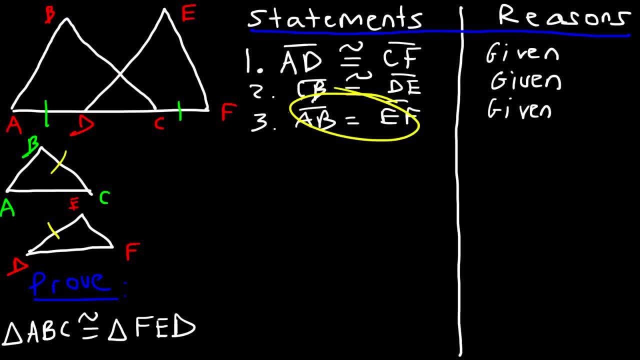 Those two sides are congruent And A B is congruent to E F. So this is A B and this is E F. So if we can prove that A C is congruent to D F, then we can prove that the two triangles are congruent. 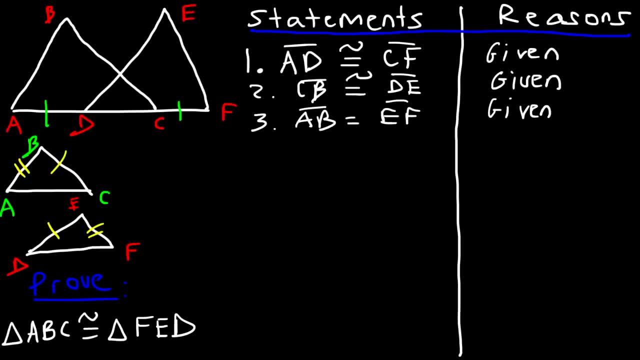 using the SSS postulate. So how can we prove that these two segments are congruent? What can we do So notice that we have an integral up in segment DC. So that implies we need to use segment addition of some sort. So first we're going to say that 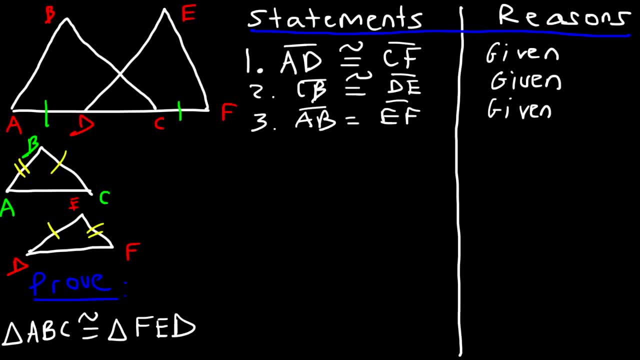 Of some sort. So first, we're going to say that AD is equal to CF before we perform some mathematical operation, And we can say this based on definition of congruent segments. Now, to get AC and DF, what I need to do is I need to 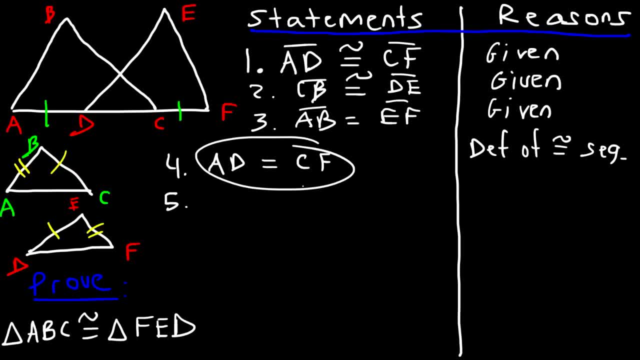 start with this sentence or this equation, and add segment DC to both sides. So I'm going to have AD plus DC and that's equal to CF plus DC. Now, because I added it to both sides, this is simply the addition property. Now notice that. 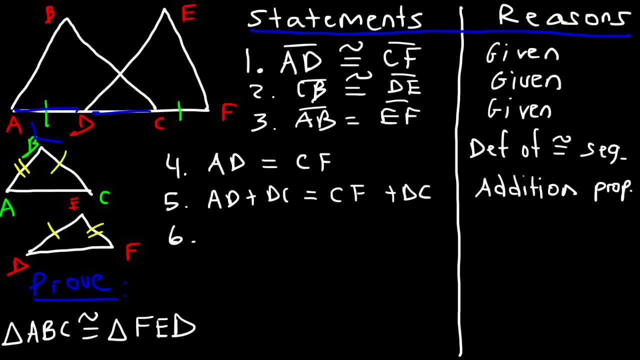 AD plus DC is AC, So I can replace the left side with AC, And DC plus CF is DF, So therefore I can replace the right side with DF, And whenever you're adding two small segments to get a larger segment, this is known as segment. 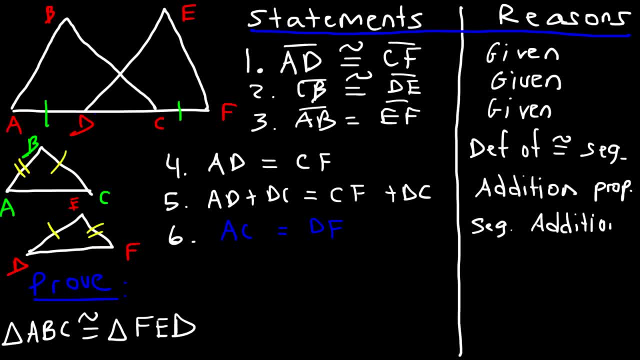 addition- Now step seven- I can say that AC is congruent to DF, And this is definition of congruent segments. So now I'm going to put the mark: This is AC and this is DF. So now we can make the final statement. 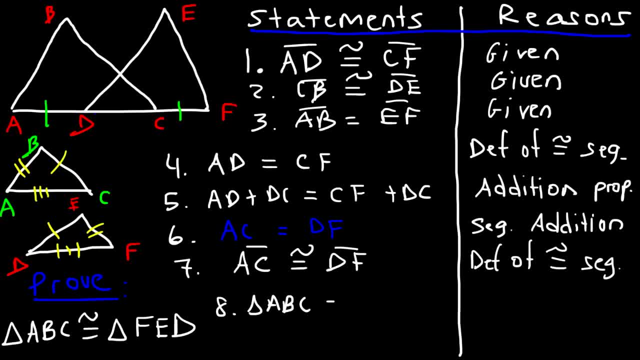 that triangle ABC is congruent to triangle F, ED, And the reason for that is the side side side postulate, And so we've used- let's see number two: CD is equal to CB is equal to DE, And we've used. 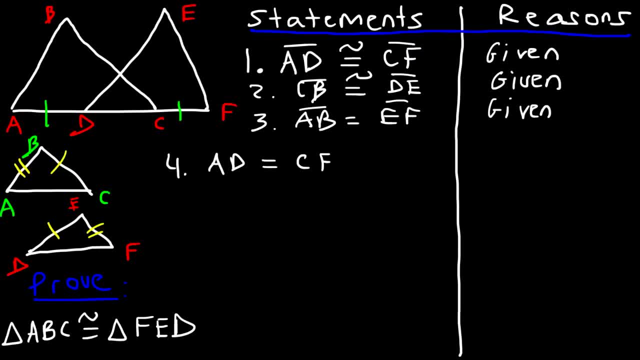 A- D is equal to C- F, before we perform some mathematical operation And we can say this based on definition of congruent segments. Now, to get A, C and D- F, what I need to do is I need to start with this sentence or this equation: 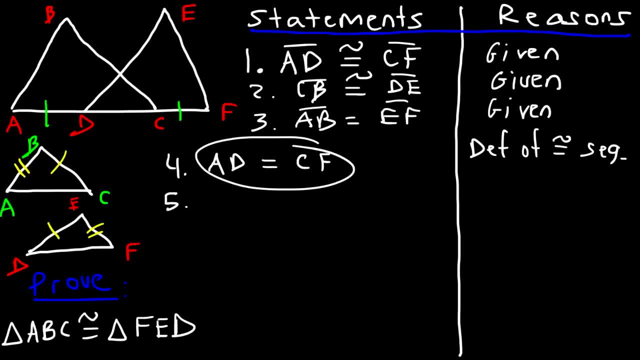 and add segment DC to both sides. So I'm going to have A D plus DC and that's equal to C F plus DC. Now, because I added it to both sides, this is simply the addition property. Now notice that A D plus DC is A C. 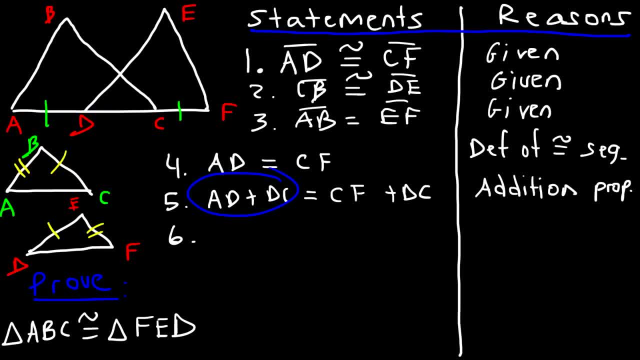 So I can replace the left side with A C And D C plus C F is D F. So therefore I can replace the right side with D F And whenever you're adding two small segments to get a larger segment. 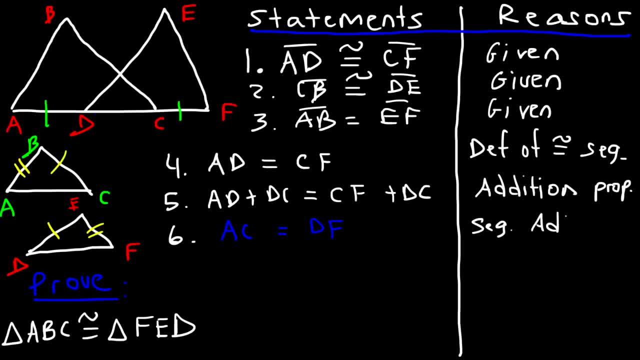 this is known as segment addition. Now step seven. I can say that A- C is congruent to D, F, And this is definition of congruent segments. So now I'm going to put the mark. So this is A C. 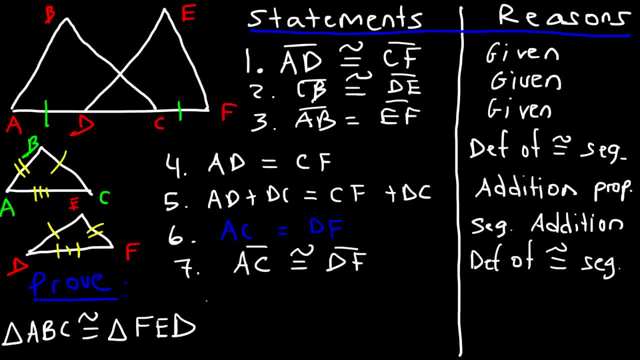 And this is D, F. So now we can make the final statement that triangle ABC is congruent to triangle F, E, D, And the reason for that is the side, side, side postulate. And so we've used: let's see: 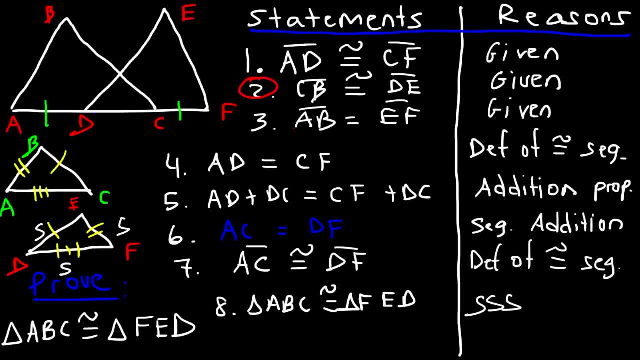 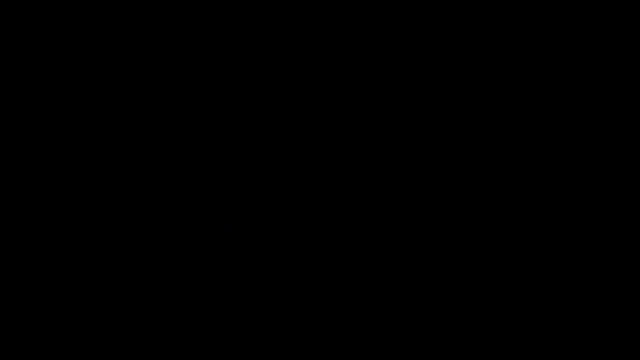 number two: CD is equal to CB, is equal to DE, And we've used number three. AB is equal to EF And also number seven. So it's two, three and seven, And that's it for this problem. Now, this is going to be. 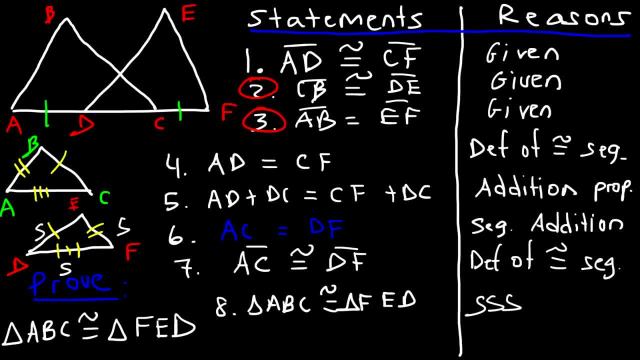 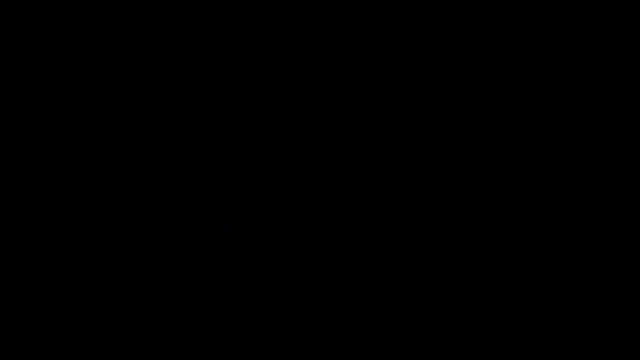 number three, AB, is equal to EF, And also number seven, So it's 2,, 3, and 7.. And that's it for this problem. Now, this is going to be the last problem of the video, So this is going to be. 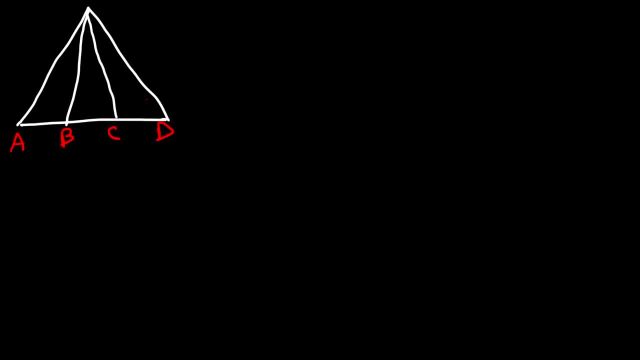 A, B, C, D and E. And so here's what we're given: We're given that B and C, that is points B and C, trisect segment AD, And then we're given that angle A is congruent. 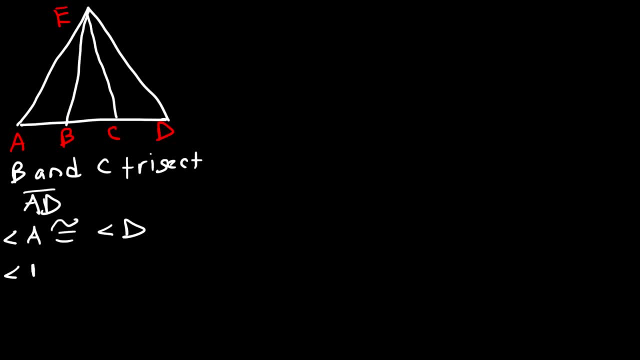 to angle D And also angle EBC is congruent to angle ECB. So go ahead and prove that triangle EAB is congruent to triangle EDC. So take a minute and work on this problem. So let's start with the first one. 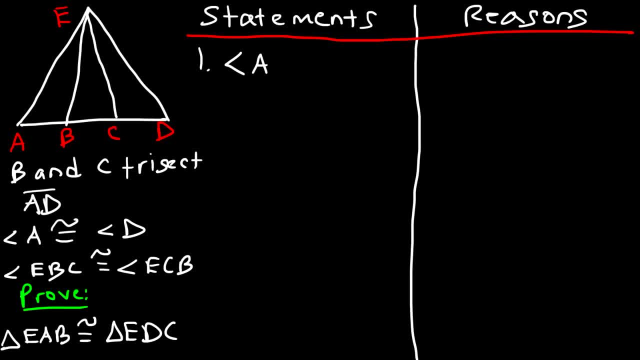 Let's say that angle A is congruent to angle D And that is given And let's mark it on the graph. So here's A and here's D, They're congruent to each other. Now number two: we know that angle. 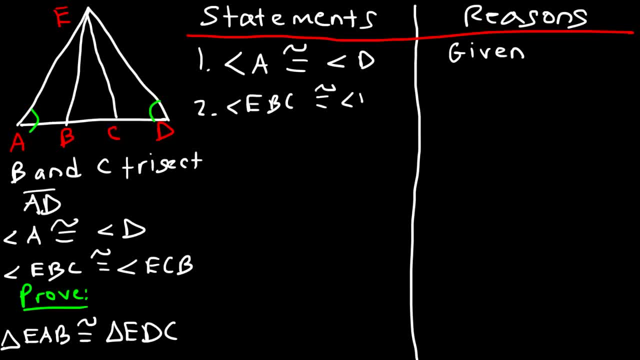 EBC is congruent to ECB, So this is EBC, So that's congruent to ECB. Let me just use a different color Instead of having so many marks. So if those two angles are equivalent, what can we conclude? Remember our 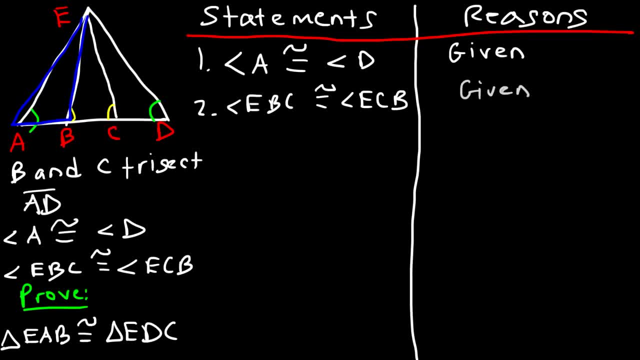 goal is to prove that triangle EAB is congruent to EDC, So we don't need these two angles. It's outside of the triangles that we want. However, we do want the angles that are supplementary to those angles, So that means that angle. 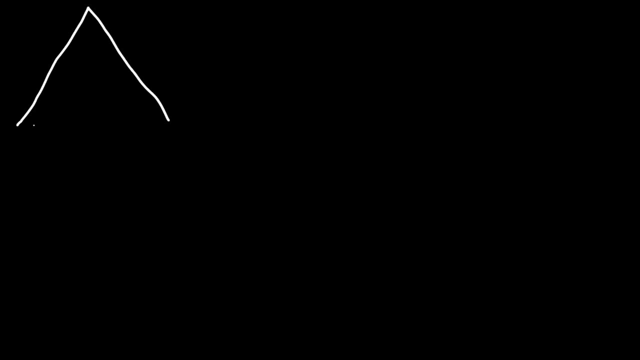 the last problem of the video. So this is going to be A, B, C, D and E, And so here's what we're given. We're given that B and C, that is, points B and C, trisect segment AD. 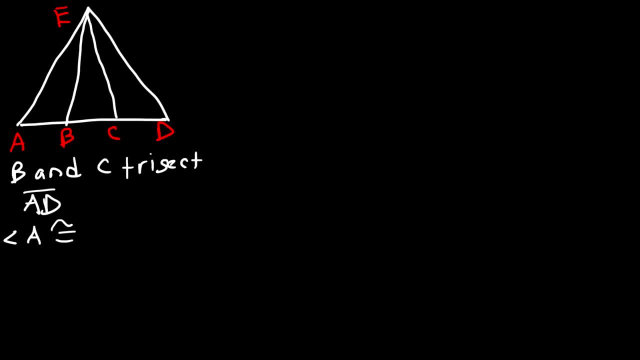 And then we're given that angle A is congruent to angle D And also angle EBC is congruent to angle ECB. So go ahead and prove that triangle EAB is congruent to triangle EDC. So take a minute and work on this problem. 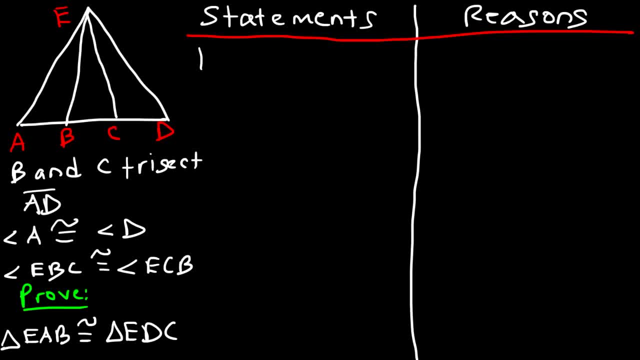 So let's start with the first one. Let's say that angle A is congruent to angle D, And that is given, And let's mark it on the graph. So here's A and here's D, They're congruent to each other. 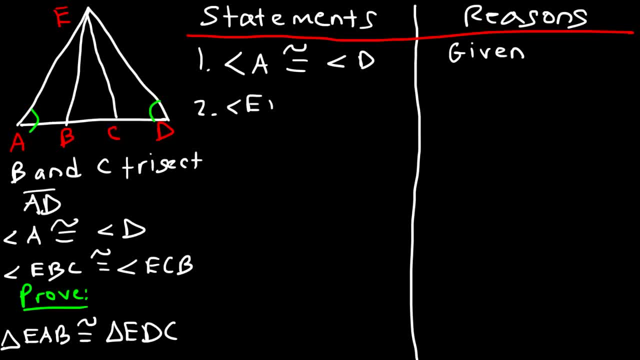 Now number two. we know that angle EBC is congruent to ECB. So this is EBC, So that's congruent to ECB. Let me just use a different color instead of having so many marks. So if those two angles are equivalent, 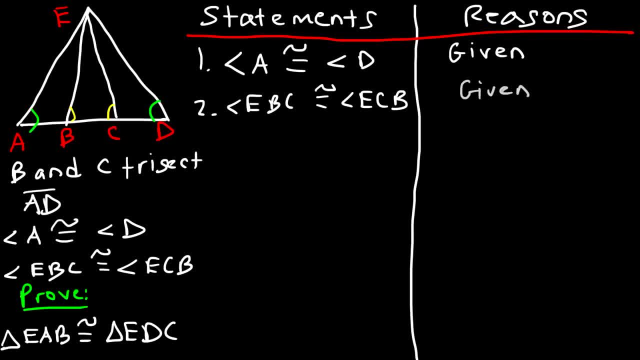 what can we conclude? Remember: our goal is to prove that triangle EAB is congruent to EDC, So we don't need these two angles. It's outside of the triangles that we want. However, we do want the angles that are supplementary to those angles. 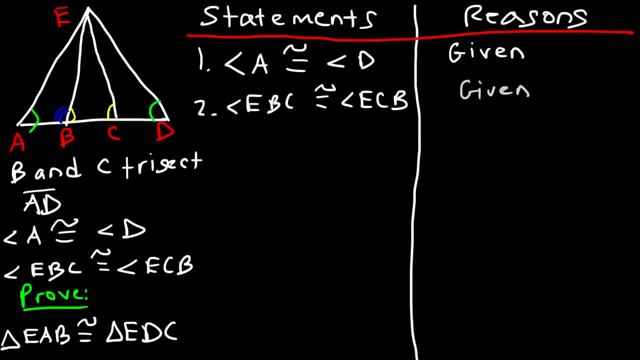 So that means that angle EBA- EBA is congruent to ECD because they're supplements of congruent angles. So let's write that Statement three: Angle EBA is congruent to angle ECD And the reason: Supplements. 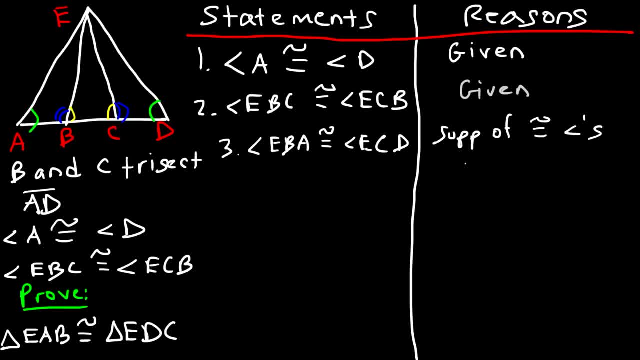 of congruent angles are congruent. Now we just need one more piece of information, And it has to do with this. So let's rewrite that statement. So, number four, Points B and C, trisect AD, So that's given. 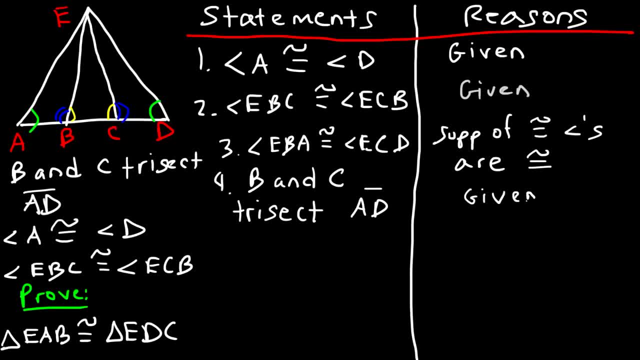 And what is the conclusion of that? Well, when something bisects a segment, it splits it into two equal parts. When you have two points that trisect the segment, it splits it into three equivalent parts. So AB and BC. 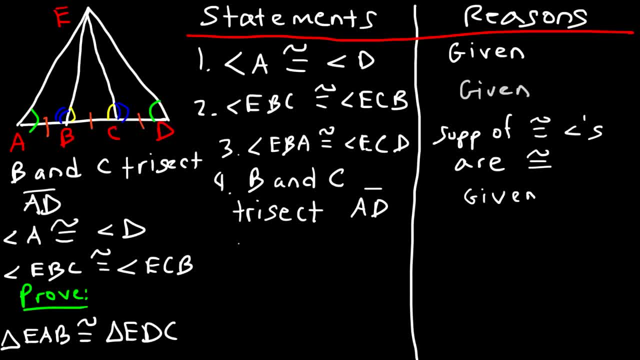 and CD are equal to each other. Bar focus. well, we can write all of it. So AB is congruent to BC, which is congruent to CD, And that's definition of an angle trisector, Or rather not an angle trisector. but 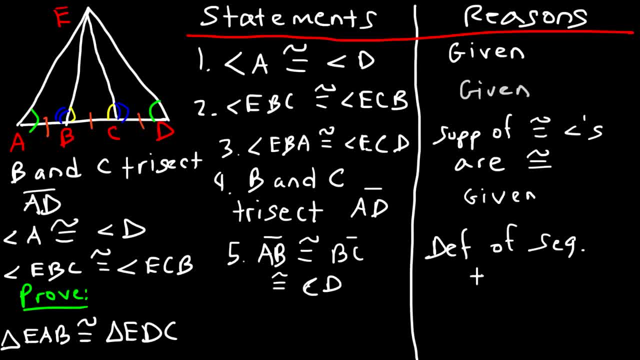 a segment trisector, Because we're trisecting a segment, not an angle. So now we have everything we need. We have an angle, a side and an angle, And the same is true for the other triangle, Angle side angle. 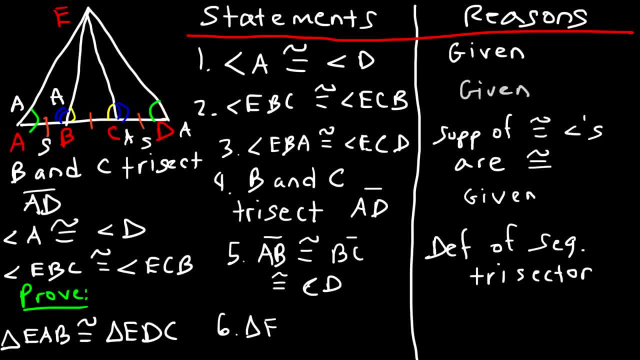 So now we can make the statement that triangle E AB is congruent to triangle EDC, And this is based on the angle side angle postulate, And we've used statement one, that is A equals D, And we also use statement three. 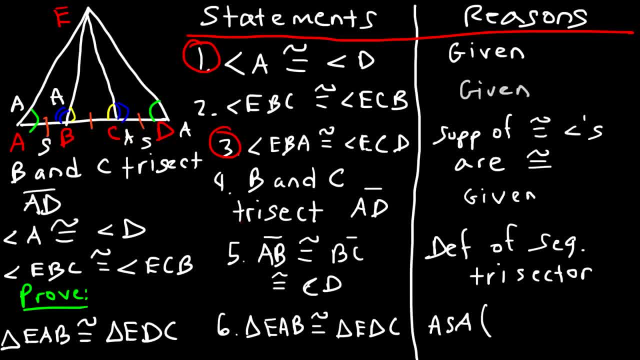 EBA is equal to ECD, And also statement five, where AB is congruent to CD. So this is one, three and five. And so now that is it. So hopefully this video gave you enough practice where you can master the ability of proving if two triangles. 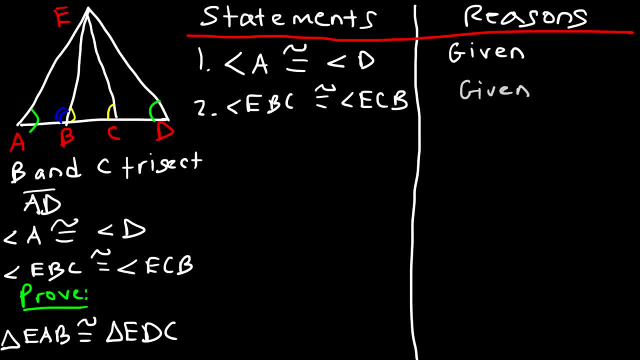 EBA is congruent to ECD Because they're supplements of congruent angles. So let's write that Statement three Angle- EBA is congruent to ECD And the reason: Supplements of congruent angles are congruent. Now we just need: 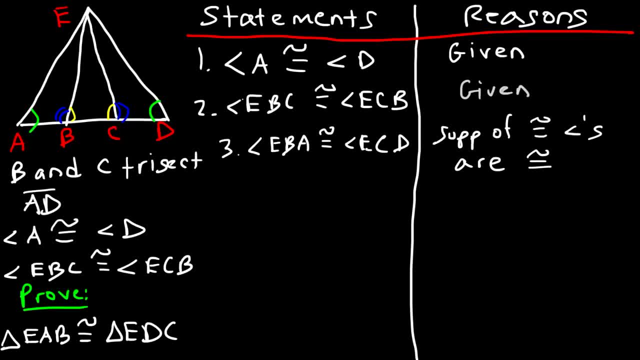 one more piece of information, And it has to do with this. So let's rewrite that statement. So, number four, Points B and C, trisect AD. So that's given. And what is the conclusion of that? Well, when something bisects, 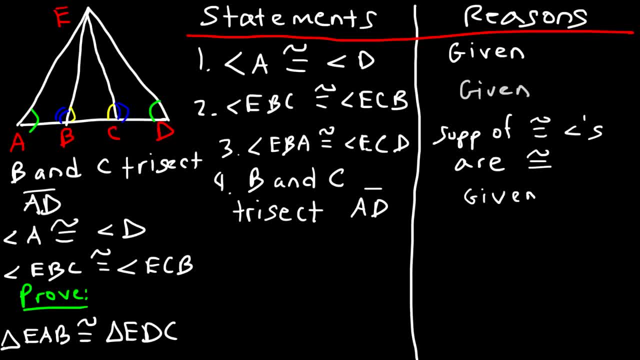 a segment, it splits it into two equal parts. When you have two points that trisect a segment, it splits it into three equivalent parts. So AB and BC and CD are equal to each other. But our focus? well, we can write all of it. 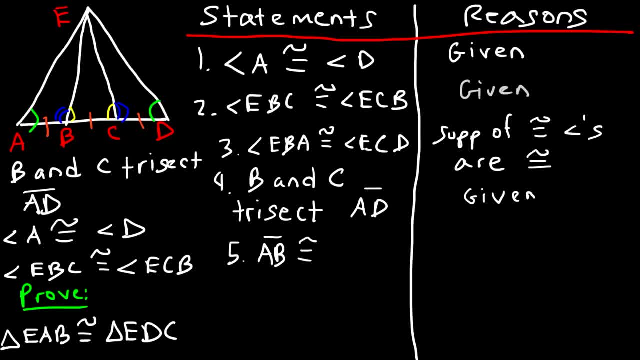 So AB is congruent to BC, which is congruent to CD, And that's definition of an angle trisector, Or rather, not an angle trisector but a segment trisector, Because we're trisecting a segment, not an angle. 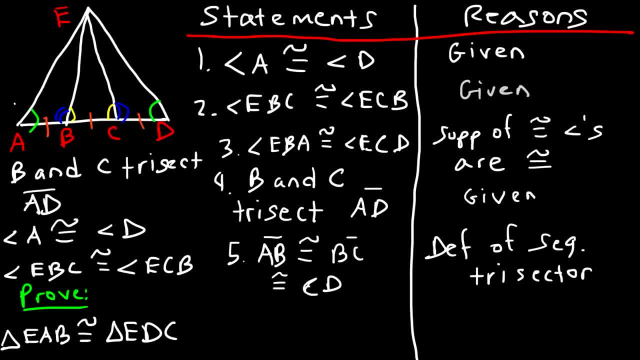 So now we have everything we need. We have an angle, a side and an angle, And the same is true for the other triangle Angle side angle. So now we can make the statement that triangle EAB is congruent to triangle. 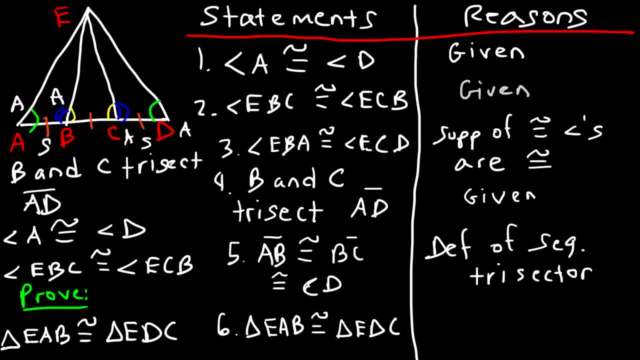 EDC And this is based on the angle side, angle postulate And we've used statement one, That is A equals D, And we also use statement three- EBA is equal to ECD- And also statement five, Where AB is congruent to CD.